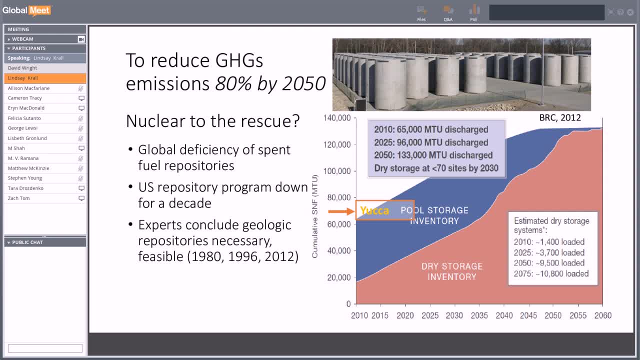 and dispose of nuclear energy. So the world's customer base is now in a state of emergency And those who have spent their spent fuel in a deep geologic repository where the safety and security risks posed by the material would be minimized- Some countries, namely Sweden, Finland and France- 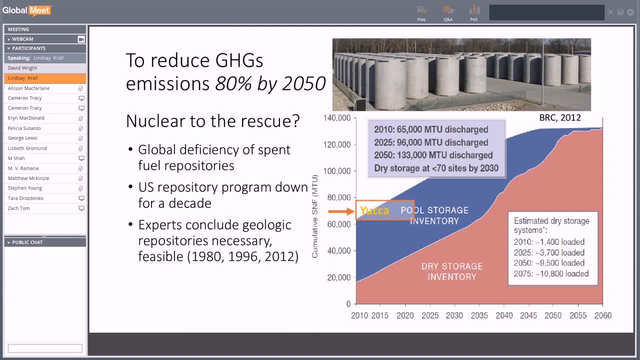 have advanced their waste management programs further than others. Here in the United States, our repository program has been down for a decade, And this has left 80,000 metric tons of highly radioactive waste spent fuel dispersed throughout the country in wet and dry storage at 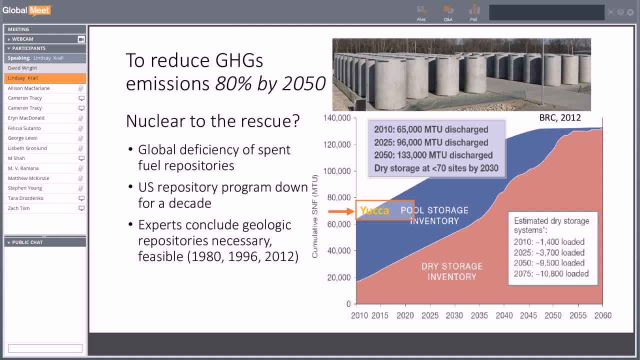 reactors that are close to retirement or that have already been shut down. Even if Yucca Mountain were close to fruition, you can see that our spent fuel inventory has already surpassed the site's legislated capacity of 70,000 metric tons. Even despite the socio-political and 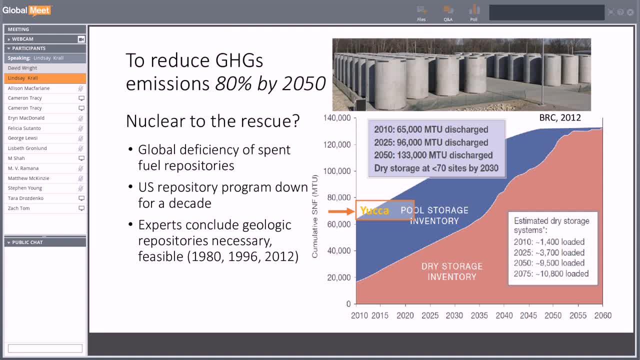 technical hurdles posed by the task of spent fuel disposal. the US Department of Energy, in 1980, the National Academy of Sciences in 1996, and the Blue Ribbon Commission on America's Nuclear Future in 2012, have independently concluded that geologic repositories are feasible. 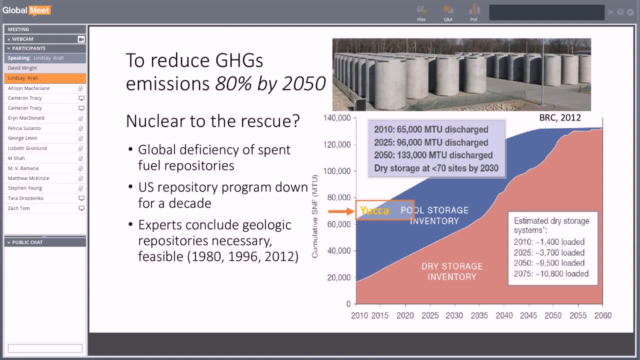 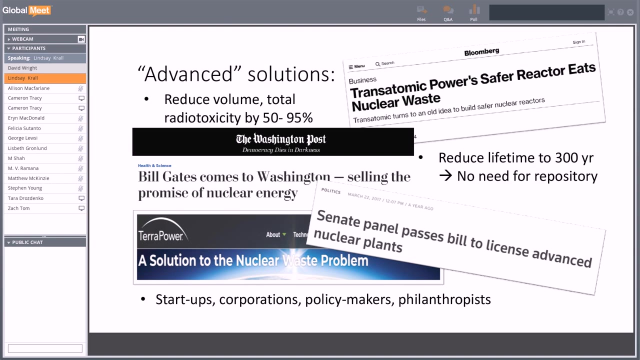 and they're necessary regardless of whether a closed nuclear fuel cycle is realized at some point in the distal future. Disposal on deep mine geologic repositories remains the international standard for securing this material, Despite the consensus among expert panels. innumerable startup companies, 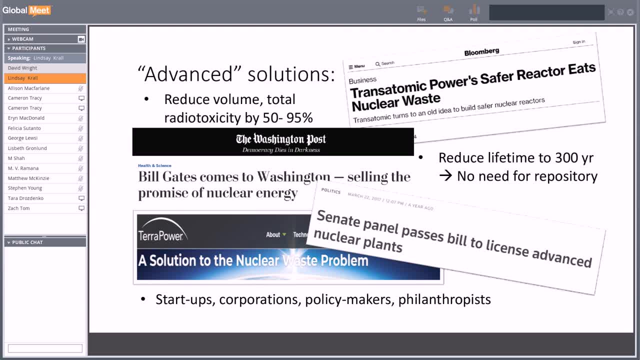 large multinational corporations, policy makers and philanthropists are standing behind generation four reactors, claiming that, with minor research and development, these would be a viable option to mitigate climate change. Among the other claim benefits pertaining to safety and security. these reactors are said to dramatically reduce the burden of radioactive waste. 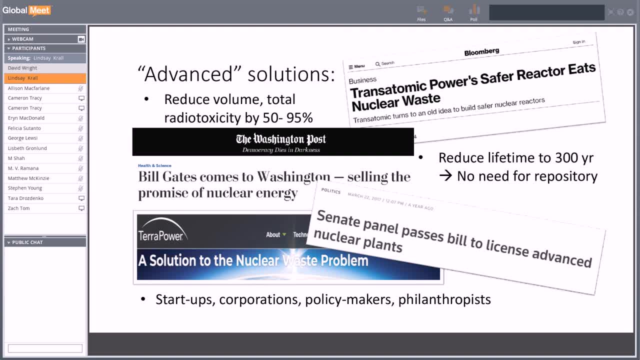 sometimes to the extent that they would obviate the need for geologic repositories. Making no comment on the RD&D efforts that would be required to deploy such a fleet of advanced reactors by 2050, we're going to deconstruct the latter claim regarding the waste reduction benefits. 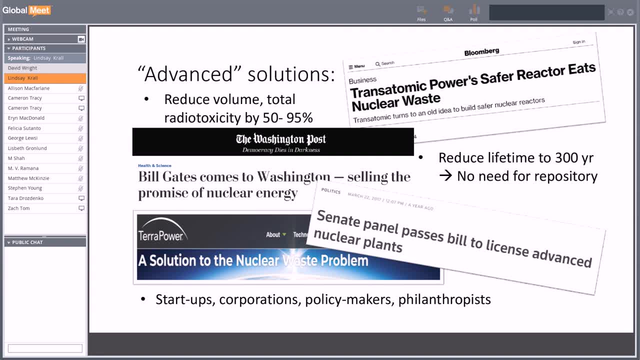 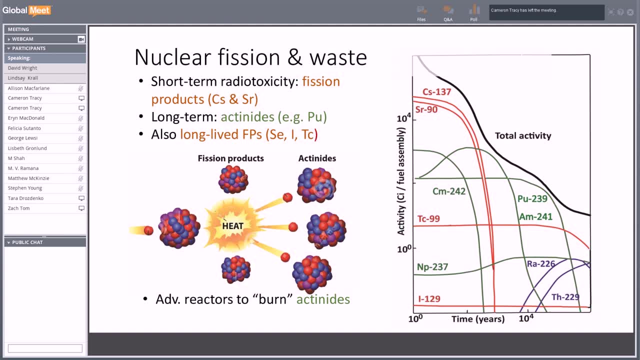 so that you can understand why these claims are grossly misleading. Sorry if this is patronizing, but it may be worthwhile to give a recap of the basics of nuclear electricity. This is derived from the heat that's released when the nucleus of an atom 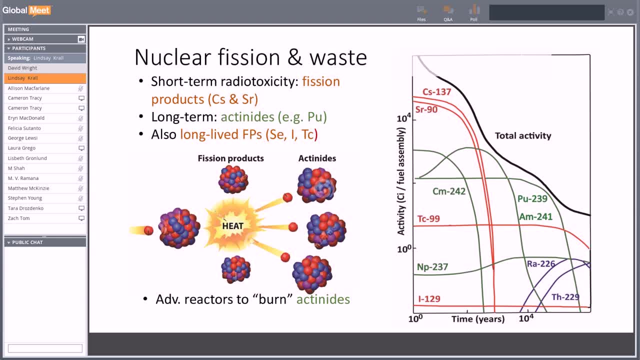 after having absorbed a neutron splits. This implicates the generation of fission products, which are two lighter elements whose mass approximates that of the fission uranium atom, In addition to two to three neutrons that may go forth to propagate the fission chain reaction. 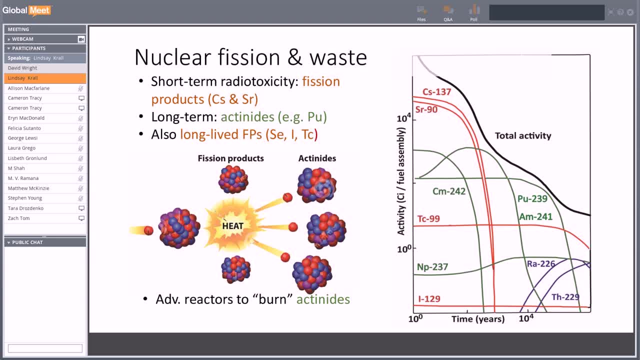 and or generate additional fissile actinides such as plutonium. So you can see that in red you have the fission products and some of them are relatively short-lived. These include cesium and strontium, which are a cause of concern. 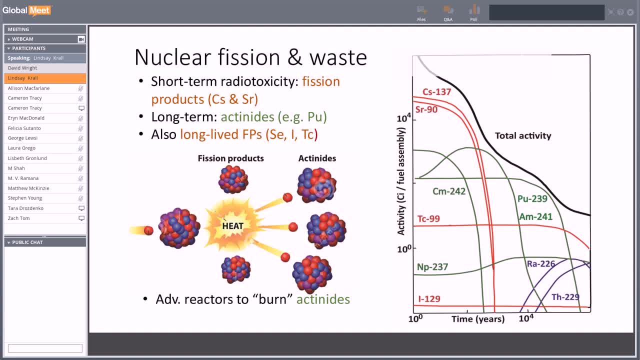 which are a cause of concern after a nuclear accident because of their very high activity. And then in the intermediate term- you could say up to say 100 or up to a million years- the actinides dominate the activity of the waste. 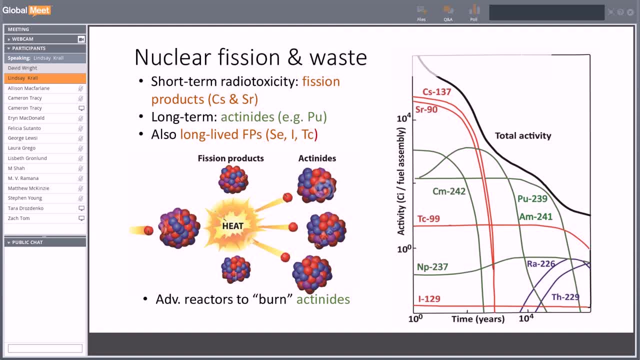 But they're also long-lived fission products. So the promise of advanced fuel cycles is to enhance the fission of the actinides which are bred in the neutron absorption reactions, so that eventually the only fission products would be destined as waste for geological repository. 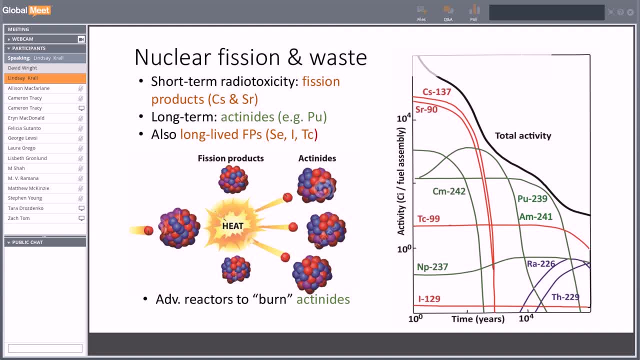 To achieve this requires that the fissile actinides are separated from the short-lived fission products, which would otherwise serve as a passive radiation barrier that would deliver a lethal dose to an intruder trying to divert the material. This reprocessing might increase the efficiency. 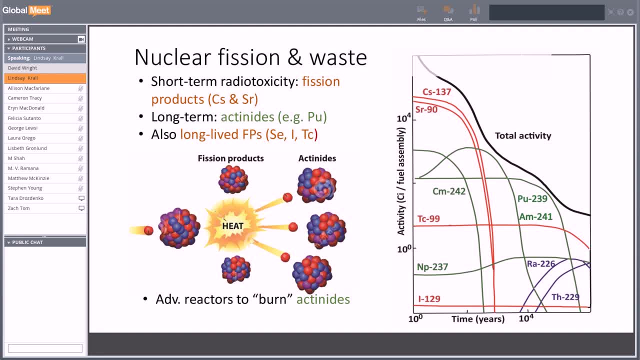 of atomic energy extraction, but it also poses a proliferation risk, in that the separated fissile material is easier to divert. All right, So you can see that if you were to remove the actinides from this decay scheme, you would have mostly cesium. 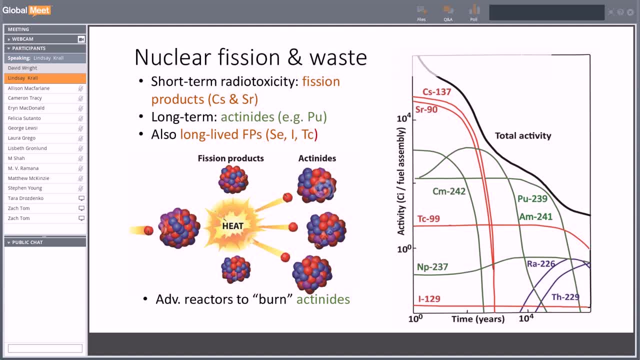 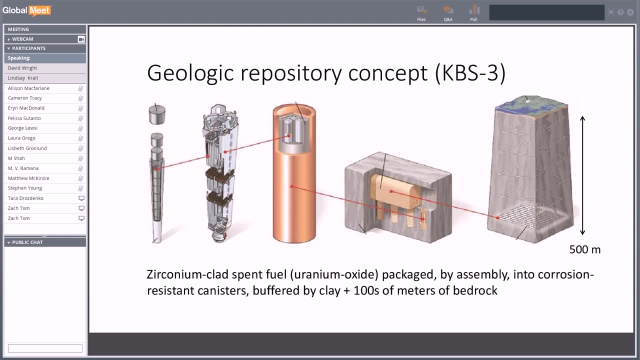 and strontium dominating the activity, and that's for approximately 300 years. So that's where this claim that advanced fuel cycles would reduce the longevity of the nuclear waste comes from. So among the nations that maintain nuclear waste management programs, the most popular 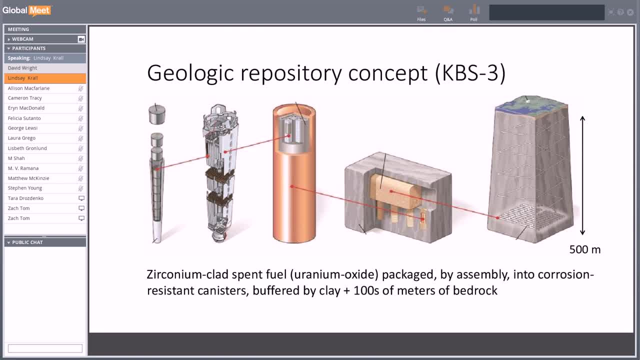 disposer concept is some rendition of the KBS3 repository, designed in Sweden. This is a multibarrier system that accounts for the array of half-lives and chemical behavior of elements present in the spent fuel. In the short term, the spent fuel. 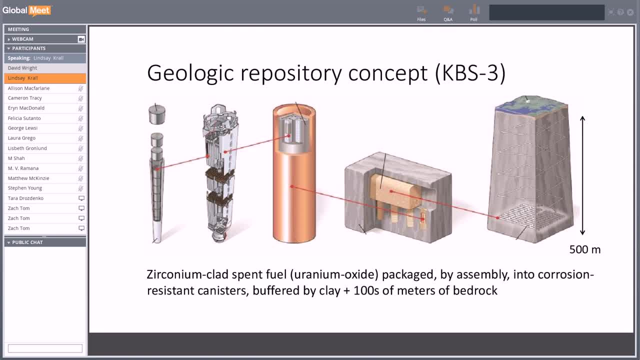 can be removed from a cooling pond and directly packaged into a canister destined for the repository, In that the spent fuel is clad in zirconium and stacked into rods that are bundled in a fuel assembly. The packaging can be done on an industrial scale. 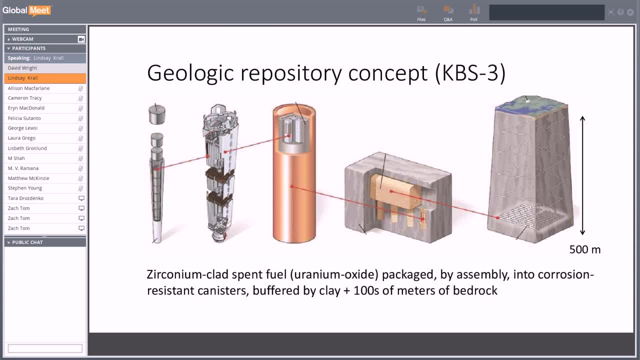 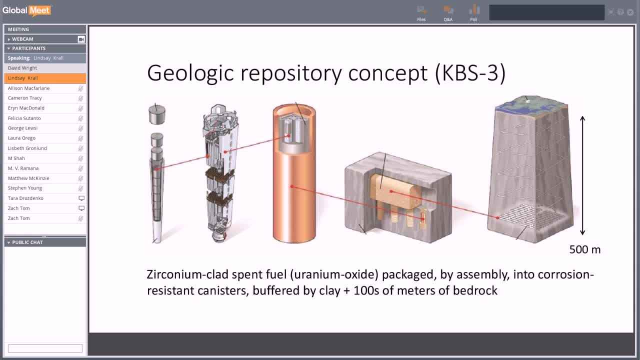 So that's where we're going with this. So that's where we're going with this. For instance, the corrosion rate of copper is very slow in an anoxic environment, such that a 5 centimeter thick copper canister should last for tens of thousands of years. 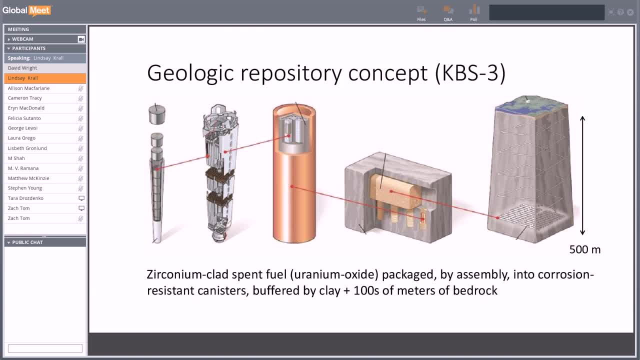 in anoxic groundwaters. This is evidenced not only by laboratory and field experiments, but by natural analogs as well. And this time horizon extends past that. And this time horizon extends past that, In case the canister fails prematurely, the repository is sited in anoxic groundwater. 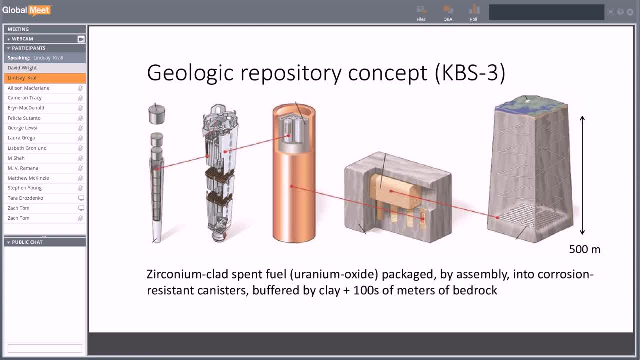 at great depths in the bedrock So that, like the canister material, the spent fuel waste form, which is predominantly uranium dioxide, is chemically stable, The spent fuel matrix having a flexible crystalline. The crystalline structure also incorporates most of the actinide elements and fission. 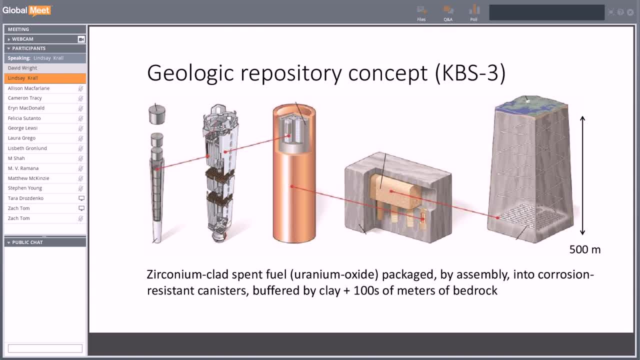 products as well through strong ionic bonding. thus dissolution rates of spent fuel and therein the rate of radionuclide released from the repository near field is slow, And the repository should be located at great depths. this one is at 500 meters, where groundwater 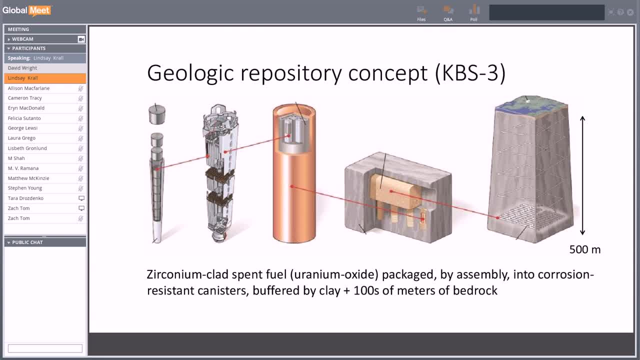 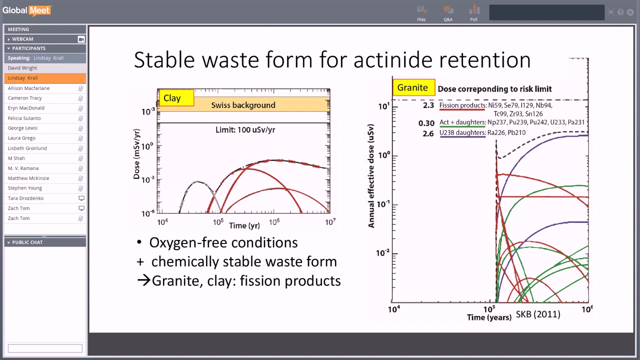 flow rates are slow and that oxygen of atmospheric origin does not penetrate the system. And this also ensures that radionuclide transport rates in the event of fuel dissolution are slow. So after a repository has an adequate multibarrier system and is sited appropriately, you can 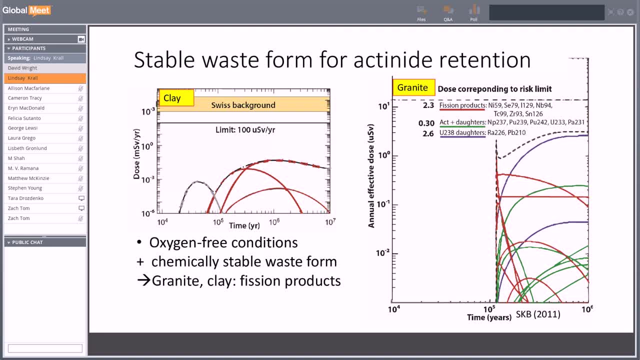 use a long-term, long-term risk assessment to determine the risk of long-term fission products. Most repository safety assessments indicate that the most significant long-term risk is actually posed by the long-term, the long-lived fission products and not as much the actinides. 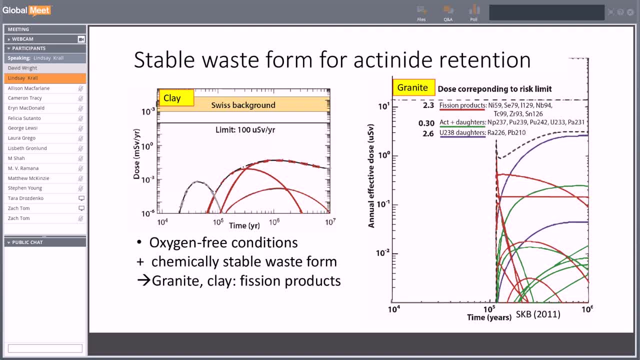 and their daughters. The daughters of uranium-238 are also released, but these exist in the same system, So you can see the 238 daughters in purple. the fission products in red and the actinides which are the lowest risk over the long-term, are in green. So the argument for burning plutonium in advanced fuel cycles seems to stem from the situation at Yucca Mountain. 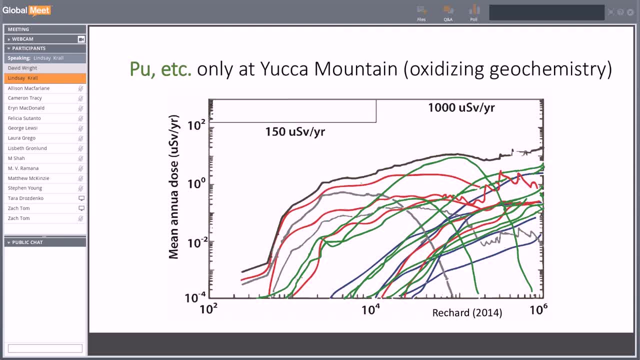 Since the now-abandoned proposed host for the US repository was cited in an oxidizing or oxygen-rich environment above a freshwater aquifer: plutonium, uranium and other actinides. 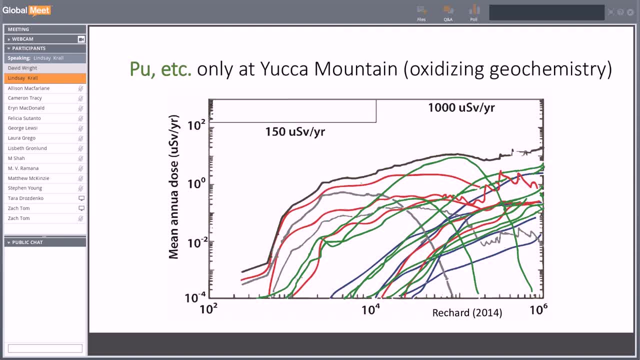 did indeed pose a risk to future populations ''. The risk was compounded with, rather than exchanged for, that of the fission products, activation products and daughters in the uranium series. But since I'm only allowing you to pose your own, un sortir x. 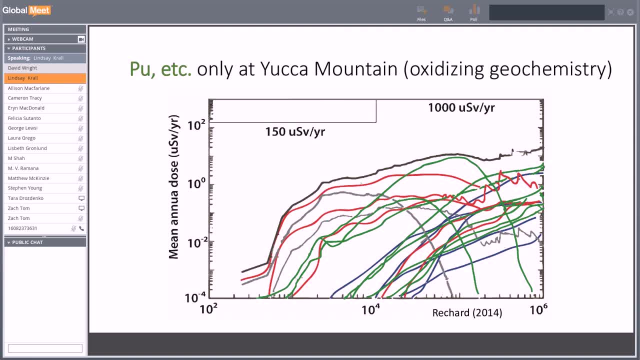 X A a, But since I'm only allotted 45 minutes for this presentation, 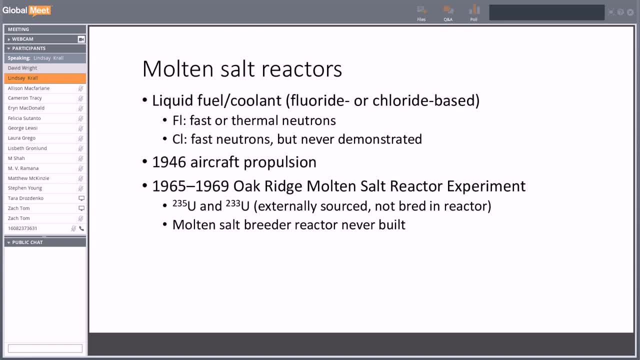 we're not going to discuss additional geologic issues at Yucca Mountain. So on to molten salt reactors. the principal difference between these and water-cooled reactors is that the designs typically call for the fuel to be dissolved directly into a bath of molten fluoride. 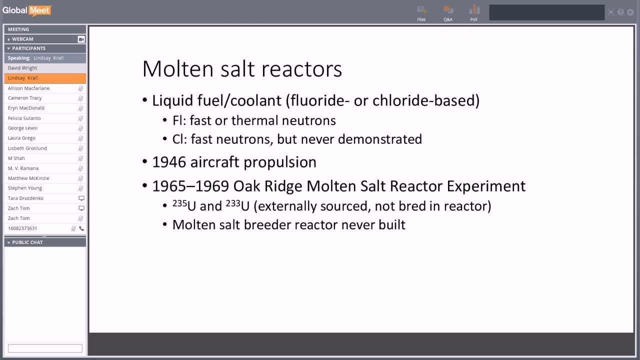 or chloride-based salt for use with thermal and fast-spectrum neutrons respectively. The reactor was conceptualized in the mid-1900s for application in aircraft propulsion, but given the radiation shielding requirements, the concept never took off, and so it was revised to meet societal demands for terrestrial energy. 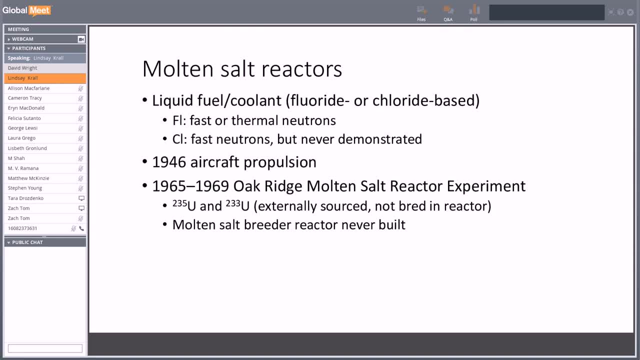 For some years. in the 1960s, Oak Ridge National Lab conducted the Molten Salt Reactor Experiment, and this showed that it was possible to fission isotopes of uranium in a bath of hot salt. but the reactor that Oak Ridge hoped would achieve the net breeding of fissile material. 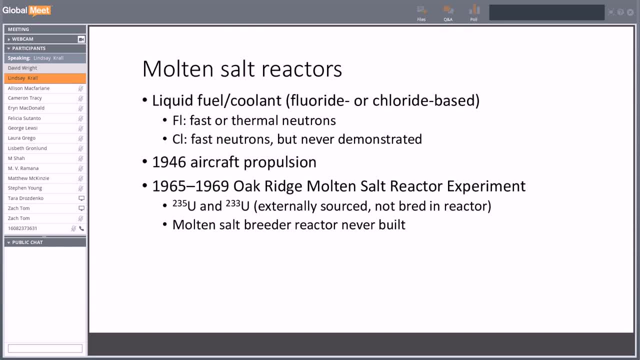 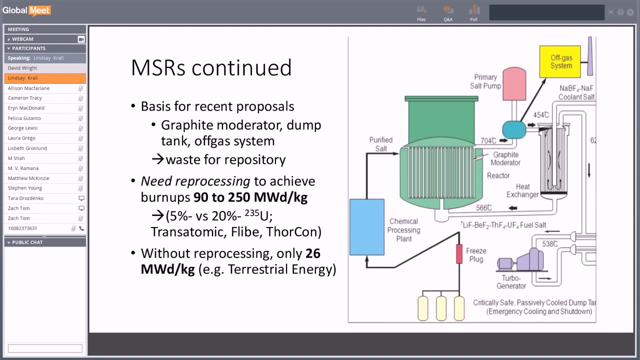 was never demonstrated in an actual reactor. So recent proposals hope to bring the breeder reactor model to life and they call for very similar systems and components as the Molten Salt Reactor Experiment at Oak Ridge. This includes a graphite moderator, a dump tank here- you can see down here. 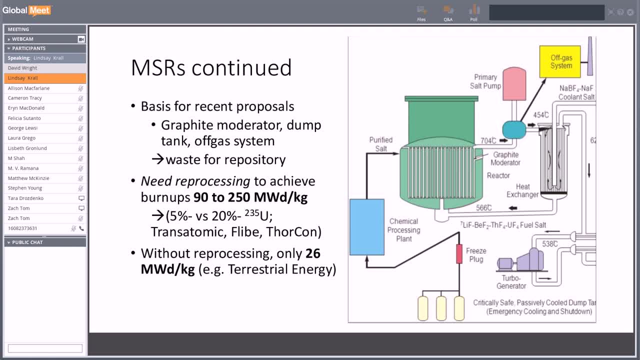 and an off-gas system which is up in the right-hand corner, Whenvening the weight of this figure. So the off-gas system is needed to vent volatile fission product poisons, including isotopes of xenon and krypton, out of the reactor pressure. 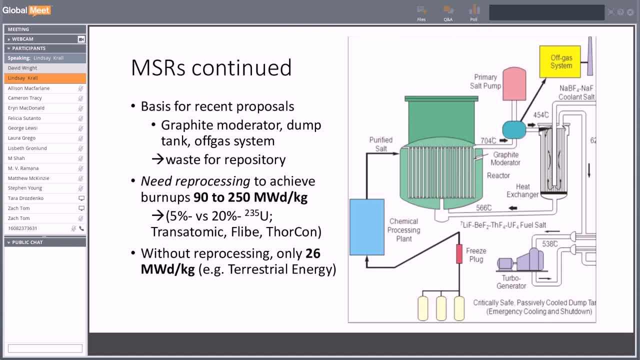 so they do not consume neutrons that would otherwise propagate fission reactions. However, as these are vented from decay and isotopes of cesium and strontium get trapped by filters in the off-gas system, it is really hard to whereby them. that is zero sec. stretching them has a high액 potential to thin them out of the reactor, for example, so that they become liquid, and then they abdicate. 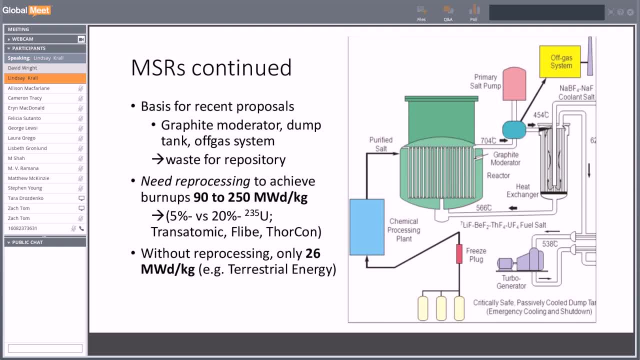 However, as these are vented from decay and isotopes are present- 두�roded- the isotopes of cesium and strontium- and get trapped by filters in the off-gas resource gas system. but those gases that do pass through the system are supposed to be collected, and 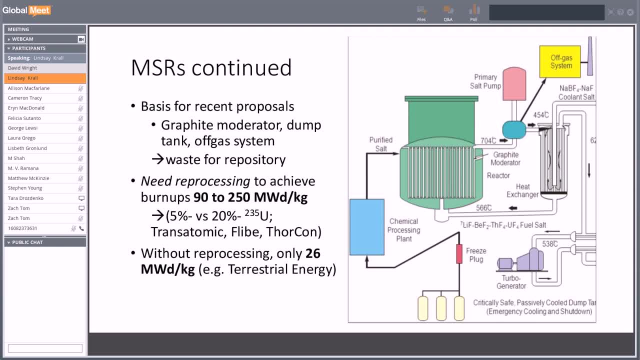 compressed into bottles, then stored and disposed of as gas. In addition to the noble gases, various other elements that are chemically incompatible with the salt migrate into the off-gas system, along with longer-lived actinides that migrate into the off-gas system because they get attached to particles of cooled salt. 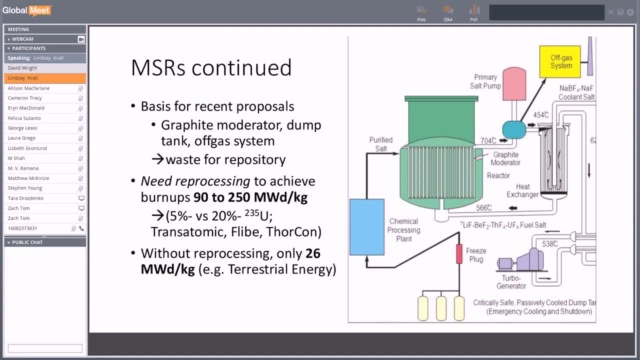 The Oak Ridge reported that these off-gas filters ultimately contained an array of short and long-lived radionuclides with a composition similar to that of high-level waste. So, considering that this contains highly radioactive material resulting from the reprocessing of irradiated nuclear fuel as dictated in the requirements, this requires geologic disposal. 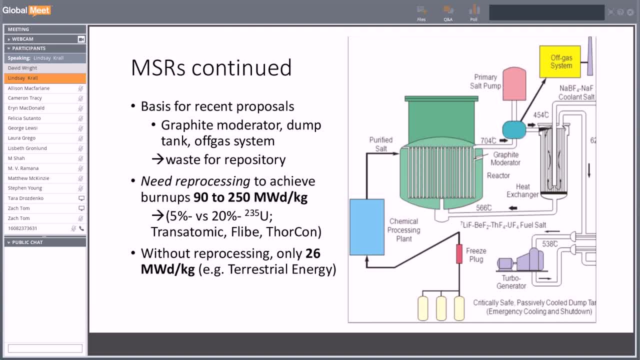 and is neglected from the waste generation estimates provided by the developers. But even given this office, In addition to these off-gas systems, molten-salt reactor designs still call for this blue box over in the left, which is a chemical processing plant. 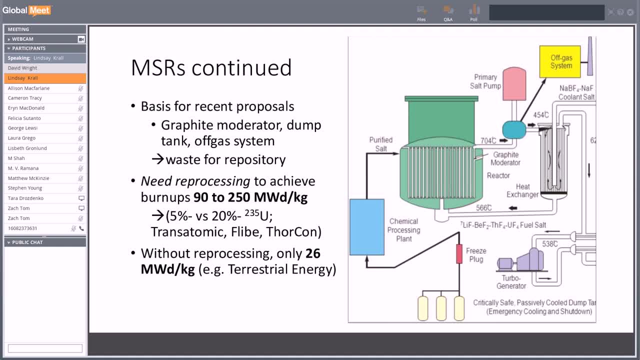 And this is either online chemical processing or at a separate facility, And only after separating fissile uranium-233 or 239 plutonium isotopes and reintroducing them to the reactor. So this is a chemical processing plant. It's a very low-duty reactor. 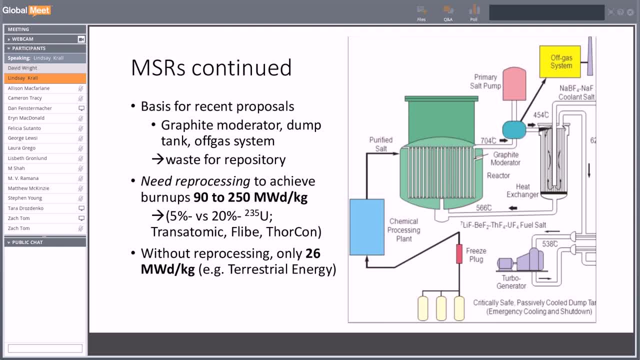 The reactor that continuously creates these fissile uranium-233 and 239 plutonium isotopes isactively regenerated to produce gas, And the person who creates these fissile uranium-233 reactors is always prepared to do the job. They are equipped with a low-duty reactor that, at least in a high temperature, can. 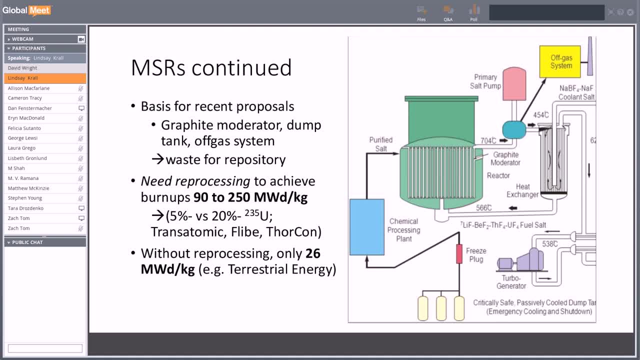 start the process And they can prepare the material for the reaction of the gas and keep it from refrigerating. And we can say that these are not cool and you have to do the work for very, very long periods of time, So they are just the typical. 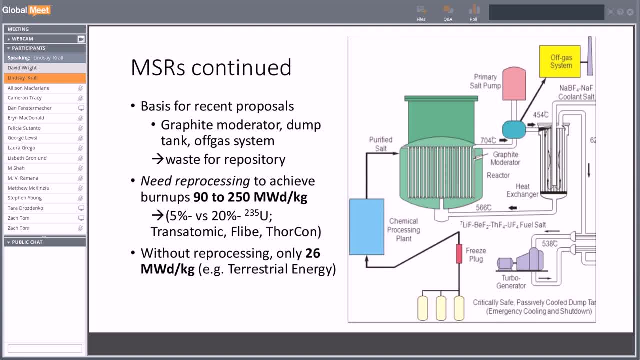 type of a reactor. There's a lot of other different kinds of reactors out there that we covered, But let's focus on the chemical processing plant. Let's talk about chemistry. Is chemistry a common currency in the United States? uranium and you forego the chemical processing, then burnups are only 26. 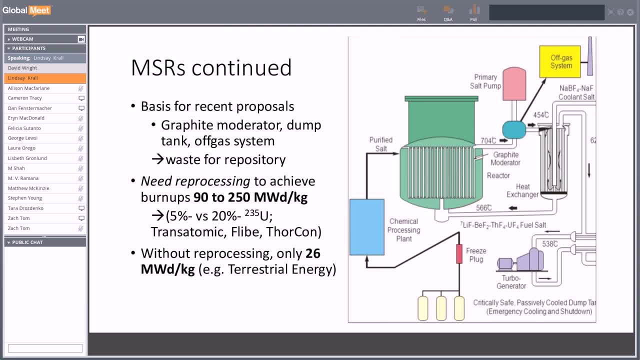 megawatt days per kilogram, which is about half that of current light water reactors. So if you're looking to compare waste generation among fuel cycles, this megawatt days per kilogram metric is inversely proportional to the mass of spent fuel produced per unit energy extracted. considering that, considering 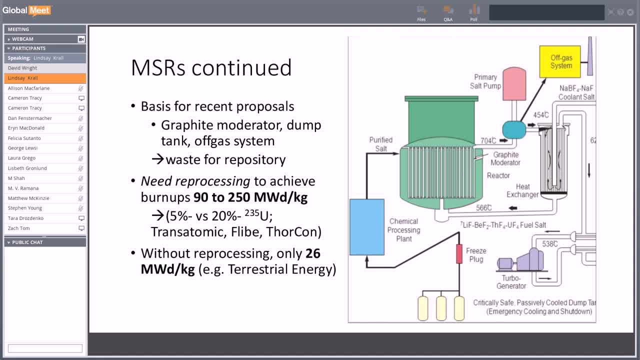 only the heavy metal and fission products for the fuel, rather than, you know, a processed waste form that's suitable for a repository. So if we're comparing apples to apples, ie a once-through fuel cycle with low-enriched uranium molten salt reactors seem to generally be the most efficient way to measure waste generation. So if you're comparing apples to apples, ie a once-through fuel cycle with low-enriched uranium, molten salt reactors seem to generally be the most efficient way to. measure waste generation. So if you're comparing apples to apples, ie a once-through fuel cycle with low-enriched uranium. molten salt reactors seem to generally be the most efficient way to measure waste generation. So if you're comparing apples to apples, ie a once-through fuel cycle with low-enriched uranium molten salt reactors seem to generally be the most efficient way to measure waste generation. So if you're comparing apples to apples, ie a once-through fuel cycle with low-enriched uranium, molten salt reactors seem to generally be the most efficient way to. measure waste generation. So if you're comparing apples to apples, ie a once-through fuel cycle with low-enriched uranium. molten salt reactors seem to generally be the most efficient way to twice as much heavy metal per unit energy generated compared to a standard. 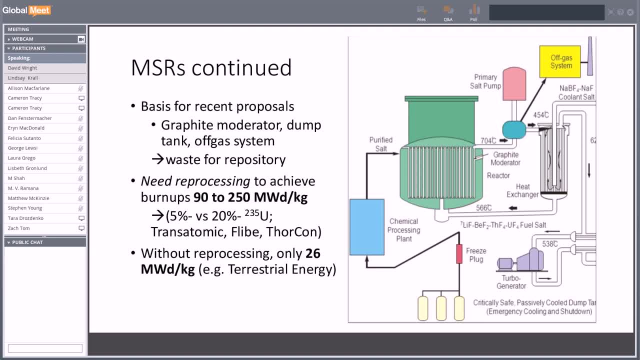 light water reactor fuel cycle. However, as previously explained, the fission product composition of the waste streams are roughly the same for each fuel cycle, regardless of burn up, And, as opposed to the mass of spent fuel, it is actually the fission products that dictate the volume and barrier requirements for most. 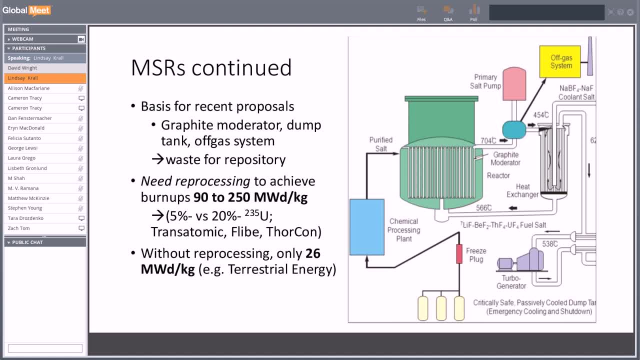 geologic repositories, with Yucca Mountain again being the exception. Fission products are the main source of heat, so they dictate the spacing of the spent fuel canisters throughout the rock volume, so that the canisters are distributed, so that the groundwater does not boil. 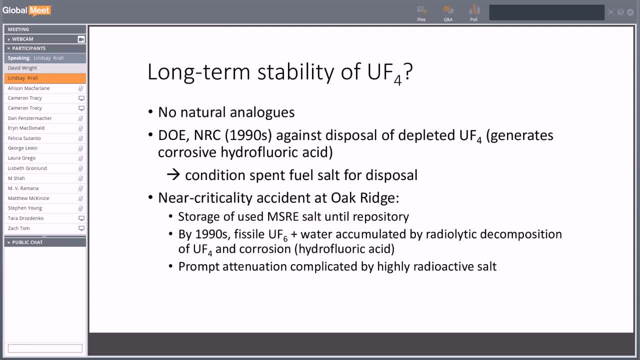 Okay. So, given that these reactors would entail significant volumes of salt in need of disposal, we would need to look for natural analogs to understand the type of environment that this material would be stable in over geologic time. But unfortunately, uranium tetrafluoride and uranium tetrachloride salts do not exist in. 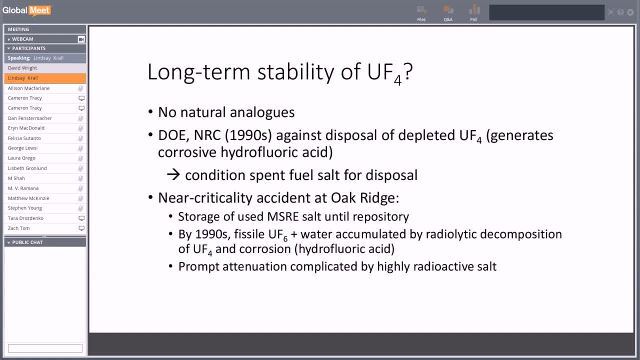 nature. This is probably because they are chemically and radiolytically unstable. One precedent regarding the disposal of uranium fluoride compounds was set in the 1990s by the NRC, who decided that the DOE should not dispose of depleted uranium in the form of uranium fluoride. 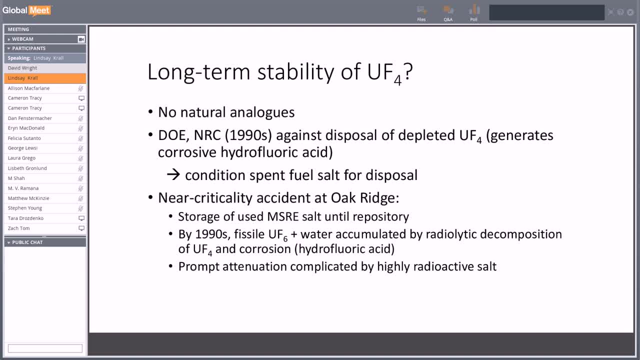 that the DOE should not dispose of depleted uranium in the form of uranium tetrafluoride. This was a relic of enrichment, so it was depleted uranium. The uranium fluoride salt dissolves rapidly in groundwater and, let's say, if one canister fails prematurely. 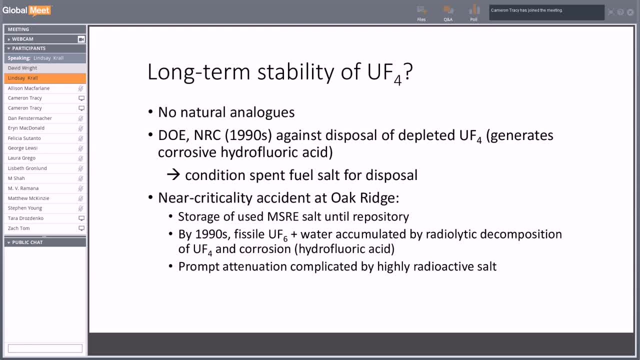 then this uranium tetrafluoride would dissolve and it would simultaneously generate hydrofluoric acid, and this acid would prompt a positive feedback loop by enhancing the corrosion of otherwise intact canisters, since the hydrofluoric acid is a very corrosive substance. 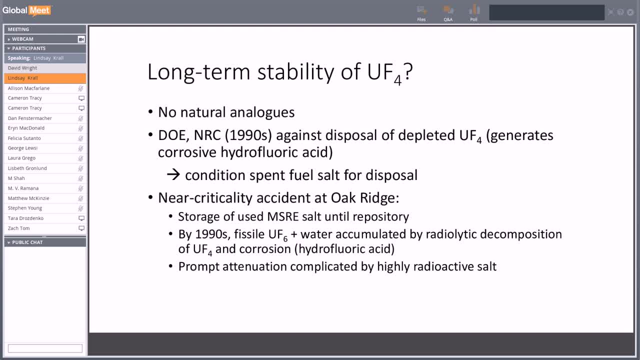 Given such issues, the near-criticality accident at the shutdown of the DOE was a very important one. It was a very important one. Molten salt Oak Ridge reactor was unexpected, but not surprising. When the experiment was terminated, the used fuel site salt was drained into those dump tanks I pointed out earlier. 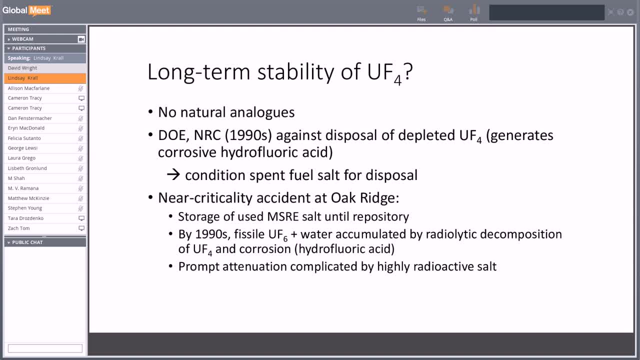 and since in these tanks the salt was in a subcritical configuration, the operators decided that it would be safe to wait some decades for part of the radioactivity to decay Before attempting to decommission the facility. However, the radioactivity can induce complex responses in materials. 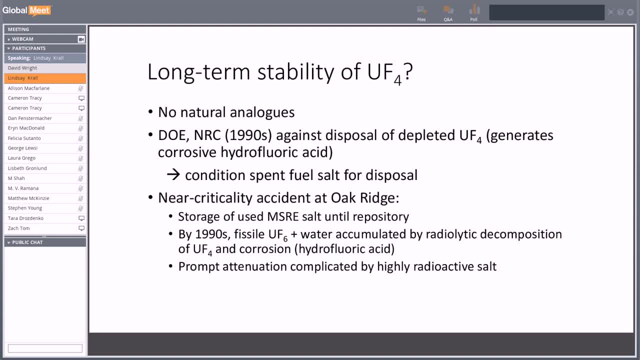 so that, as the radiation damage accumulates, the chemically bonds are weakened. The bonds in uranium tetrafluoride, being very weak, were eventually broken by the subatomic particles flying around in the tanks and this caused the generation of uranium hexane. 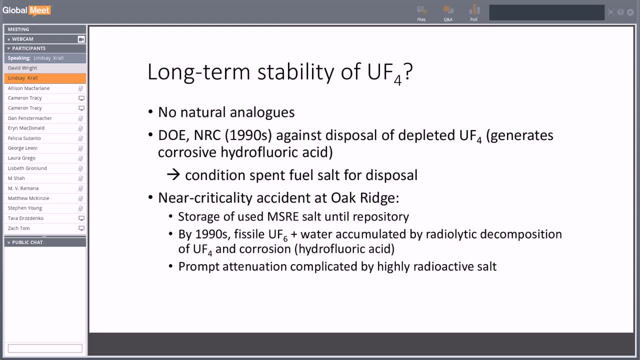 and this caused the generation of uranium hexafluoride and fluorine gas to form, the former of which accumulated in sections of the off-gas system. Maintenance engineers recognized that uranium hexafluoride was being lost from the tanks and that this was enriched in fissile uranium-233,. 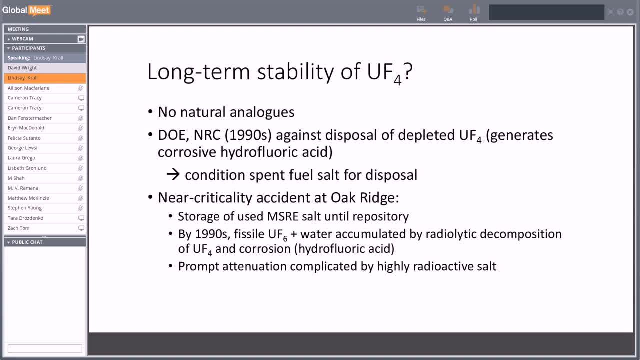 but as long as water wasn't present to moderate a fission chain reaction, it was presumed that this would be acceptable. However, the uranium hexafluoride and fluorine gas that formed in the tanks, the fluorine gas, interacted with moisture in the dump tanks. 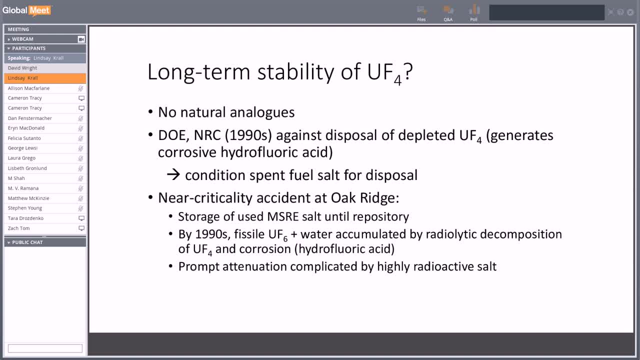 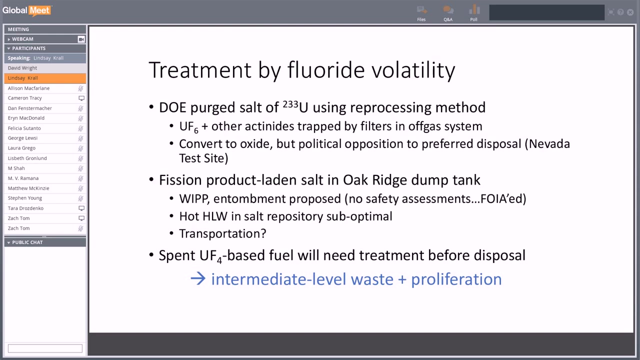 and so this formed hydrofluoric acid and corroded the pipes and allowed more water to ingress. Given the remarkable safety risk posed by this situation, it required prompt attenuation. so it was complicated by the high radiation fields emitted by the salt and the influence of the fluorine gas on the energy source. 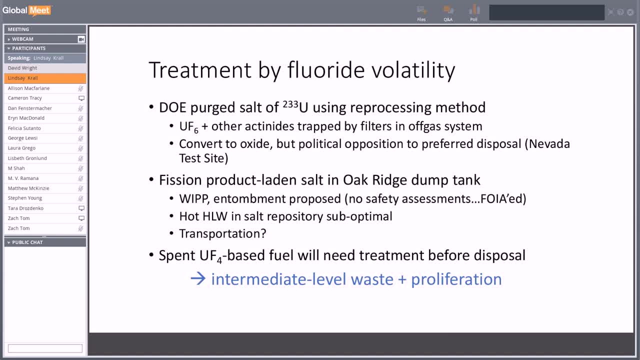 was by bubbling fluoring gas through the system. This formed a volatile uranium hexafluoride that could then be trapped by filters in the off-gas system Conveniently. this approach, or the fluoride volatility method, is the same that it was in the first place. 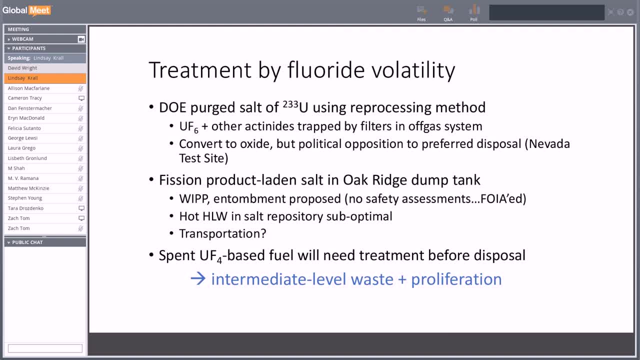 and this is why we had to change and change the process. So we have a problem that we have to solve. All right, and is once again being proposed for the reprocessing of used MSR fuel salts, so that its fissile material can be separated and reused. 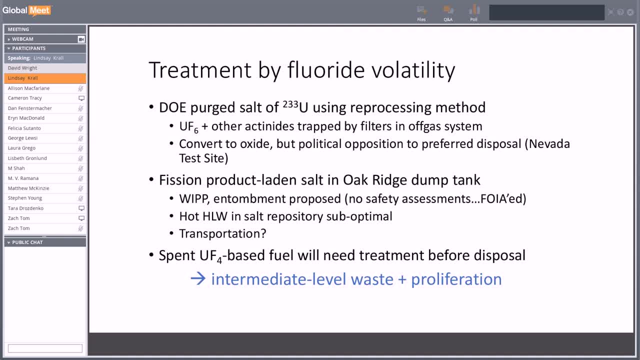 Since, having extracted the uranium, the DOE has converted it to uranium oxide, probably mixed with depleted uranium, and suggested that it be sent to the Nevada test site and disposed of as low-level waste, despite its classification as special nuclear material. As for the fission product, lead and sludge in the Oak Ridge dump tanks, it's still 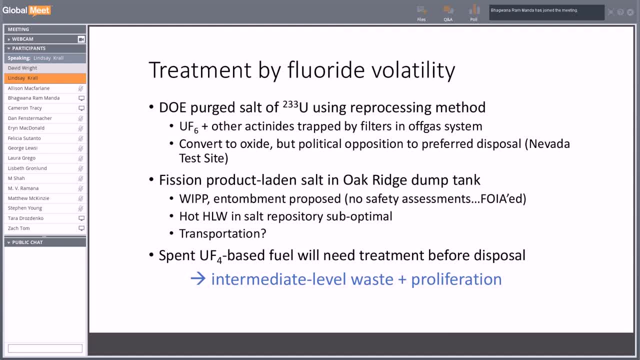 there. It's not really clear what the DOE plans to do with it. Sending the tanks to WIPP and on-site entombment have both been proposed. Do you want to say what WIPP is, in case people don't know what WIPP is? 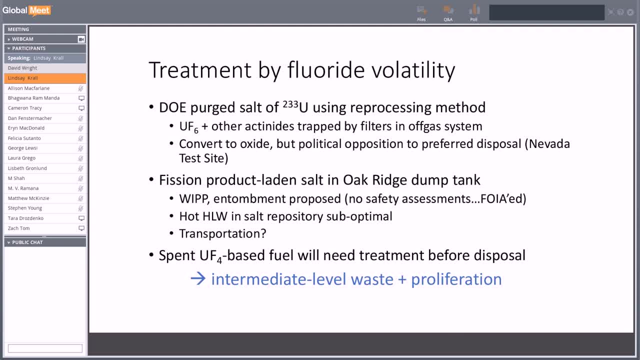 Oh, WIPP is the Waste Isolation Pilot Plant in New Mexico. It's an intermediate-level waste repository that the DOE operates. Okay, but the details regarding either of these options and the implicated feasibility and safety aspects have not been shared with the public. Hopefully. 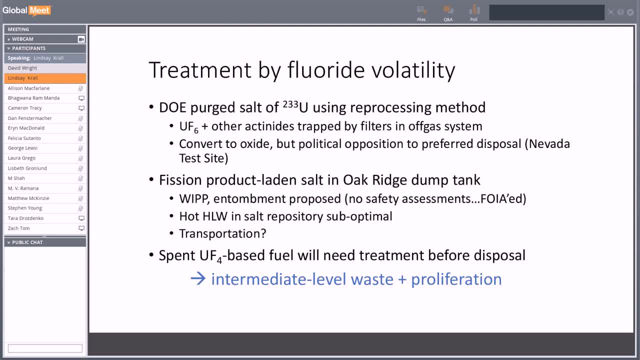 my Freedom of Information Act request will provide some more details there. To put the experience at the Molten Salt Reactor Experiment in perspective, this was an 8-megawatt reactor which is orders of magnitude smaller than the MSR designs being proposed today. 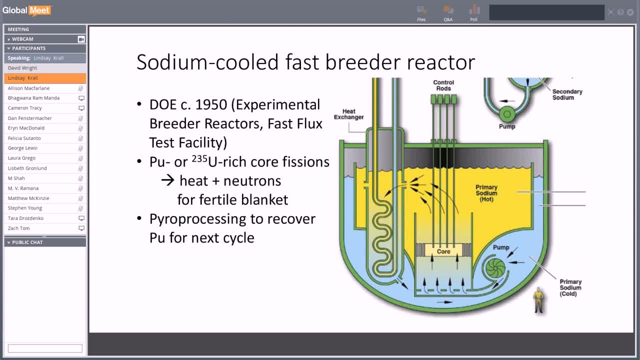 And under the second most popular Generation 4 design on the market. the Sodium Fast Breeder Reactor is another concept that dates back to the early 1900s or to the early 1950s. The DOE operated three such fast reactors and today plans to build another similar. 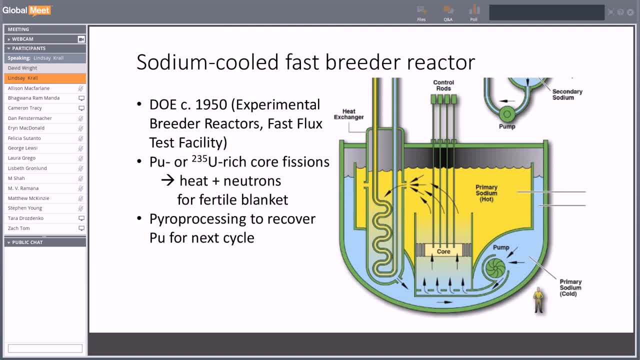 test reactor in Idaho. This reactor calls for a core that is enriched typically up to 20% in fissile material, being plutonium-239 or 235 uranium. This is supposed to fission and produce heat plus neutrons. In addition, the DOE has a core that is enriched with plutonium-239, which goes forth to generate 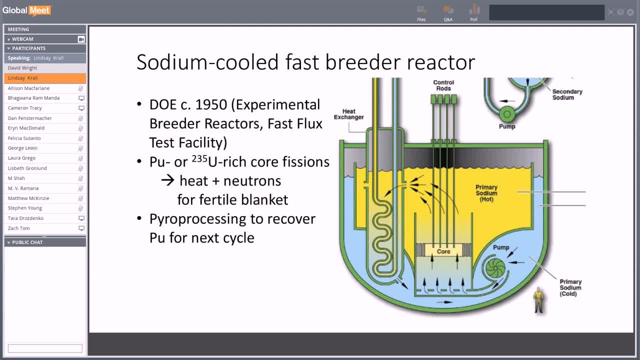 239 plutonium in a blanket of 238.. The bred fissile material is then processed, often through an electrochemical approach called pyro-processing, then eventually purified and used to refuel. the core. Developers suggest that the pyro-processing systems be co-opted. 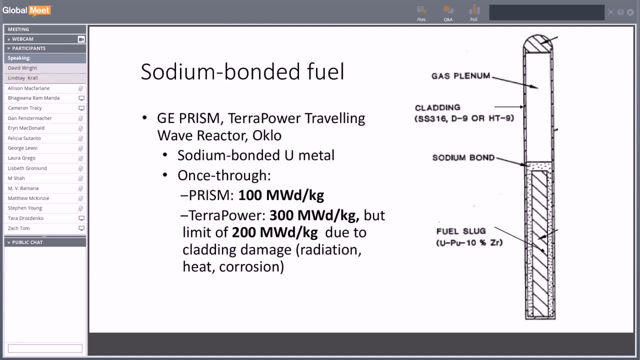 with the reactor. Unlike the Molten Salt Reactor, the Fast Breeder Reactor fuel prints are not directly dissolved in the sodium coolant. Rather, most of the designs promoted by US companies call for sodium-bonded metallic uranium fuel. This was developed during the late DOE Liquid Metal. 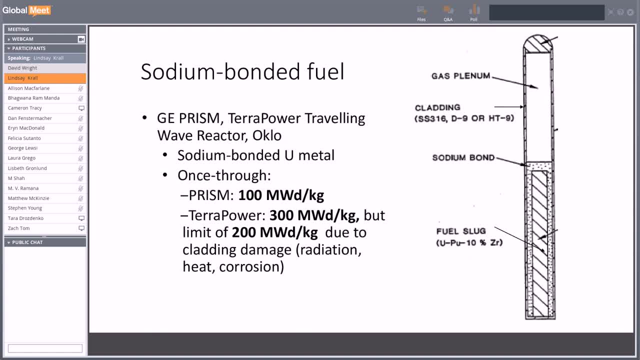 Fast Breeder Reactor program. Here you have a diagram of the fuel and you can see that it was hand-drawn several decades ago. This is clad by stainless steel as opposed to zirconium, but designs in the rest of the world typically call for MOX fuel rather than metallic uranium fuel utilization. 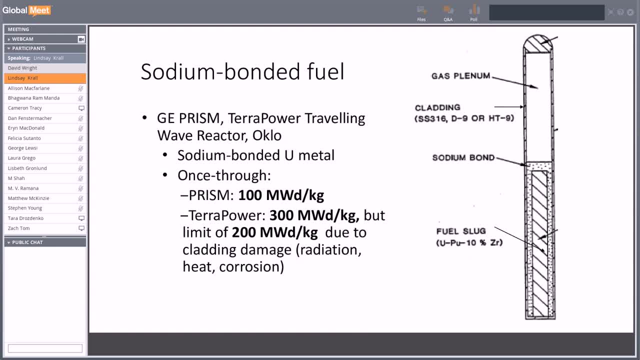 However, DOE posits that the sodium-bonded metallic uranium fuel can be used as a fuel fuel. However, DOE posits that the sodium-bonded metallic uranium fuel can be used as a fuel fuel. However, DOE posits that the sodium-bonded metallic uranium fuel can be used as a fuel fuel. 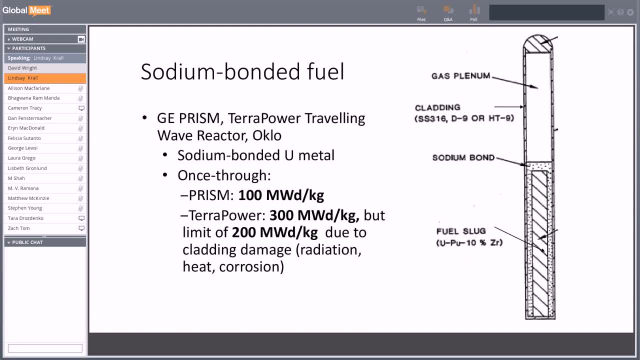 If any agent comes into contact with the BBT of the fuel, that's when saturated sodium, bonding products or explicitly less chemical reactions are applied. Another old example is49 Burning금. Burn Burnups in a once through fuel cycle in theory are higher than for whitewater reactions. 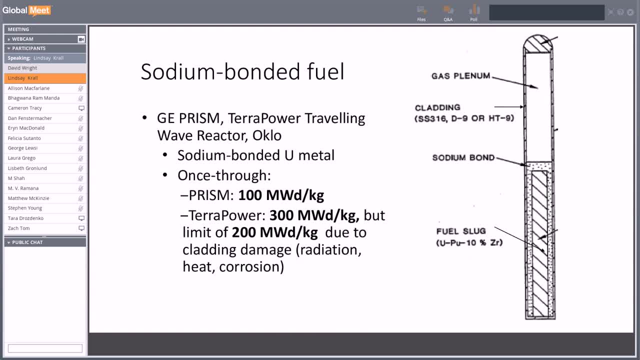 This is would be explained in patients who only go for high doses light water reactors. TerraPower is hoping to exploit such a once-through fuel cycle, wherein the blanket, after having bred sufficient plutonium, would be shuffled inward without needing to be reprocessed. Neutronic simulations indicate that burnups of 300 megawatt days per 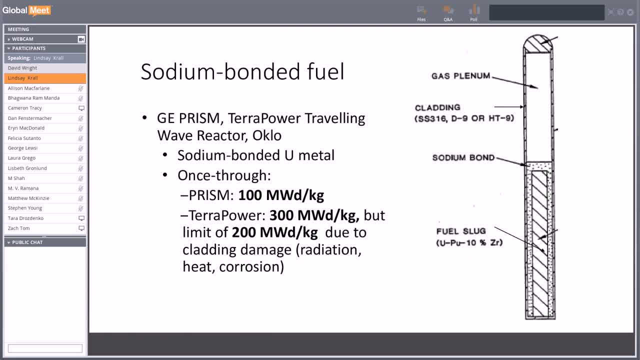 kilogram might be achieved if high assay, low enriched uranium is used for the initial core loading. But among the technical challenges associated with the design, the fuel cladding in such a fuel cycle would be damaged before such high burnups are reached. It's a very extreme. 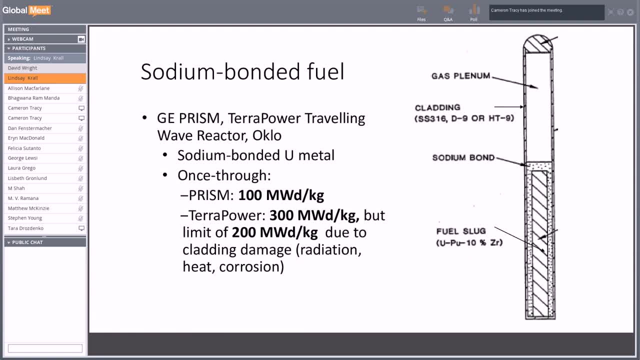 environment with fast neutron radiation. Damage by fast neutrons also heat and corrosion. So given the mechanical limits to the cladding burnups of 200 megawatt days per kilogram might be more realistic, according to experience at the DOE test reactors. 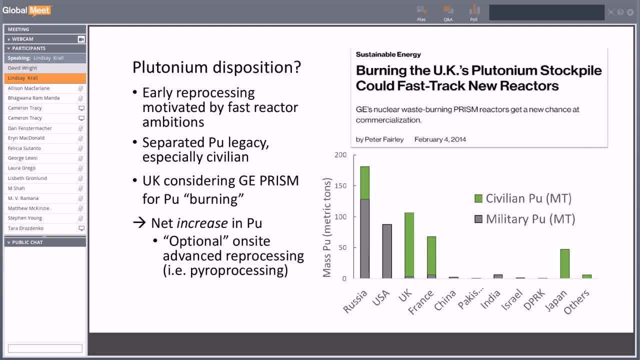 Compared to thermostats, thermal neutron reactors. fast neutron reactors can breed and fission plutonium more efficiently. So energy security rules of the mid-1900s motivated the development of these plutonium fueled reactors because uranium resources were thought to be scarce. 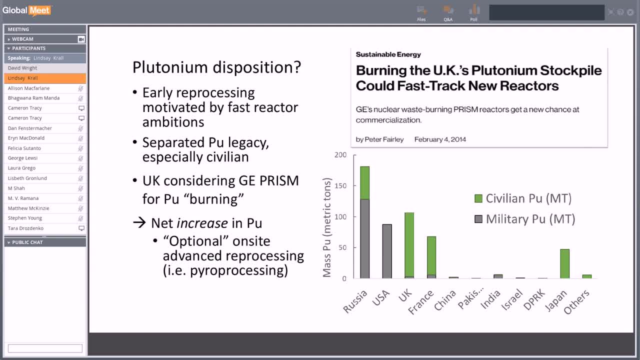 Many nuclear countries began reprocessing the fuel from their water or graphite-moderated reactors so as to stop the production of plutonium. So, in the mid-1900s, the development of plutonium pile, plutonium that could be used to fuel a future fleet of fast reactors. But given that 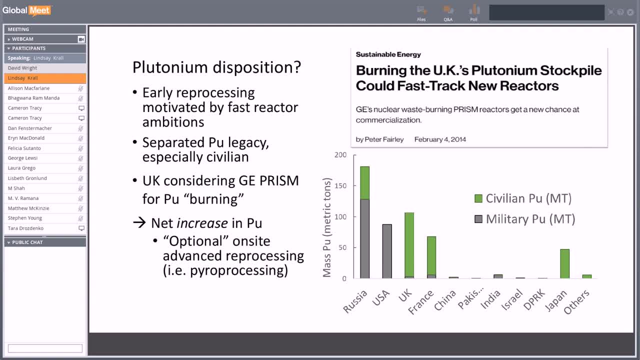 abundant uranium was soon found, that nuclear energy was not as widely adopted as anticipated, and that the development of fast reactors was plagued by issues such as sodium fires. there now exists a legacy of separated civil plutonium, which is weapons usable and has no 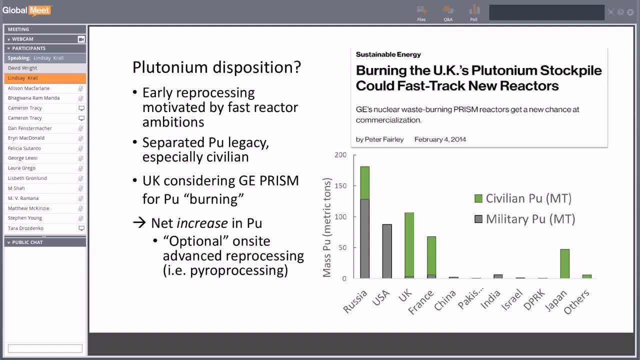 passive radiation field to secure the material from intruders. The issue is particularly acute in the United Kingdom, who has been considering to utilize the unproven GE prism technology to fission this separated plutonium. GE Hitachi has suggested that the reactor can be used in a 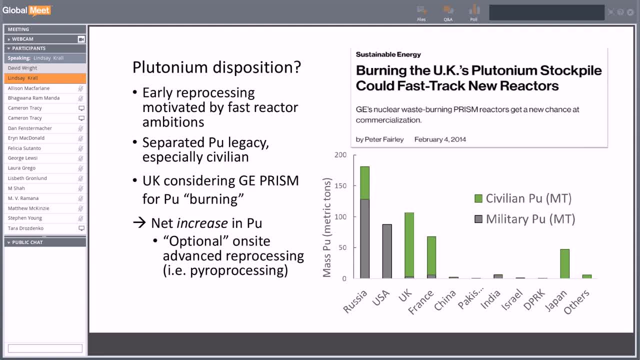 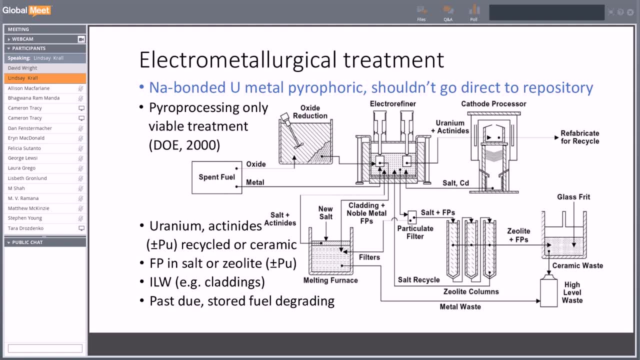 fuel cycle to burn the plutonium, Although such a scheme would actually generate a net increase in plutonium. Furthermore, it's not clear that this reactor can be utilized in a once-through direct disposal fuel cycle. In decommissioning the experimental reader reactor, 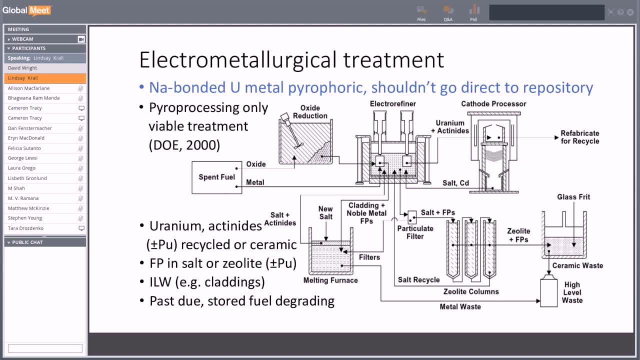 Idaho National Lab set a precedent with important sodium-bonded waste management implications. The material is classified as pyrophoric in that it reacts violently if exposed to water. Thus, the spent reactor fuel cannot be directly disposed of in a geologic repository, The DOE. 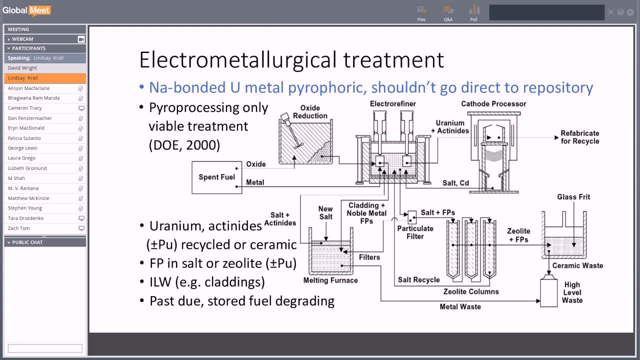 decided that the only way to deactivate the fuel was through electrometallurgical treatment. This calls for the same systems as pyro-processing, except that a slight modification is made to electrolyte salt used in the process. So this is a very involved process. You can see a lot of. 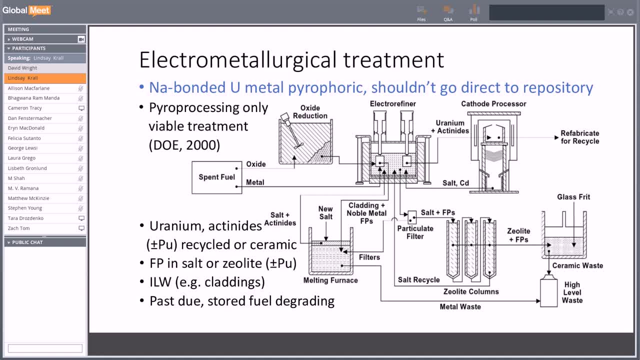 components become contaminated along the way, and so all of this would be considered intermediate level waste. As is typical for reprocessing operations, DOE is decades and billions of dollars behind in treating the experimental fast reader reactor waste. Foyer documents recovered by Ed Lyman indicate that, meanwhile, the spent fuel in wet storage is. 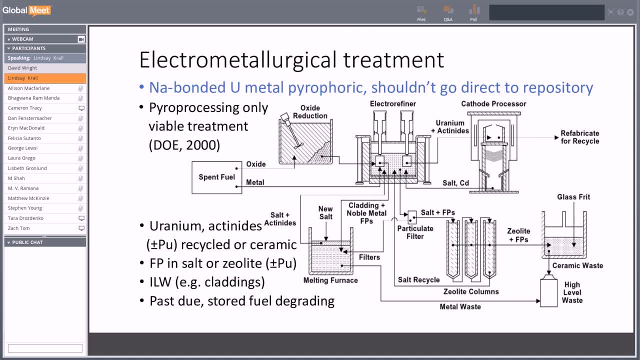 degrading in at least one way. So a lot of different processes in the DOE process. In at least one case, the fuel showed that a pyrophoric reaction had occurred between water and the metallic fuel element. This was following corrosion of the stainless steel cladding. 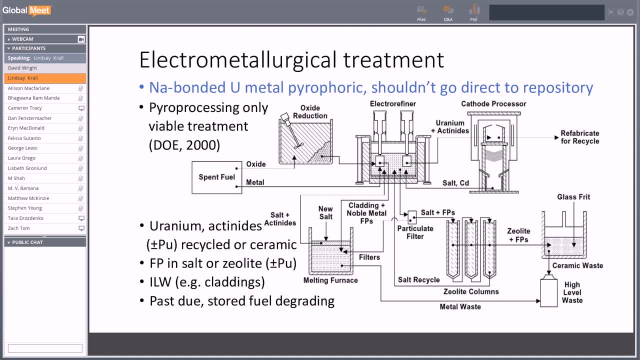 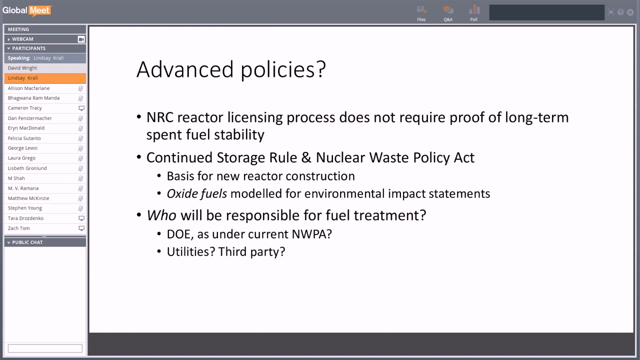 So it seems that the waste is literally burning. The notion that this technology is needed simply to prepare sodium bonded fuel for disposal has proliferation implications, as well as implications for exporting a technology that can easily be modified to separate fissile material. So, concerning advanced policies for this, 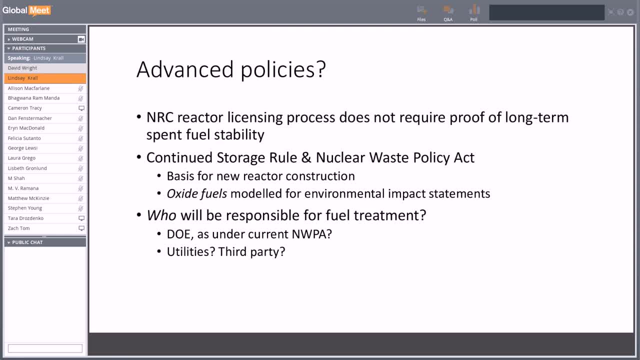 there's always a complaint that reactor licensing is entirely favored for light-water reactors, And it does seem to be true that the licensing process is light-water reactor specific, in that there's no requirement that the developers need to approve that the spent fuel is light-water. 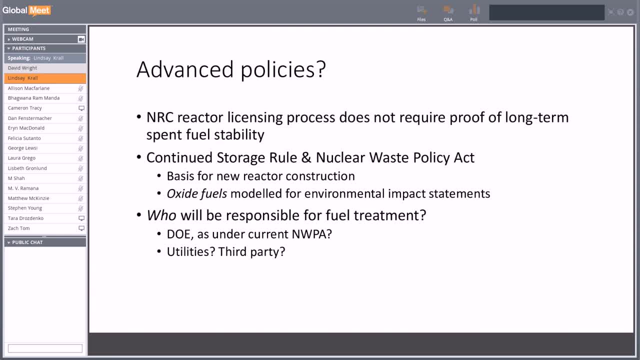 This is because the spent fuel is long-term, is stable over the long-term time period. There's really no long-term requirements on the spent fuel at all in the reactor licensing process. However, we do have the Continued Storage Rule and the Nuclear Waste Policy Act. 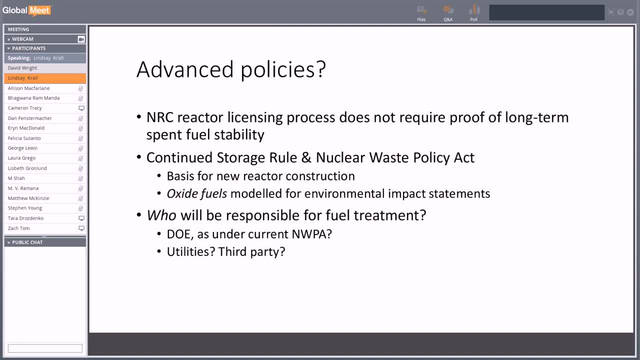 These form the basis for new reactor licensing, reactor construction. the continued storage rule says that the spent fuel is safe as stored on the surface until a geologic repository becomes available, and this was decided in the context of the cancellation of the Yucca Mountain project. 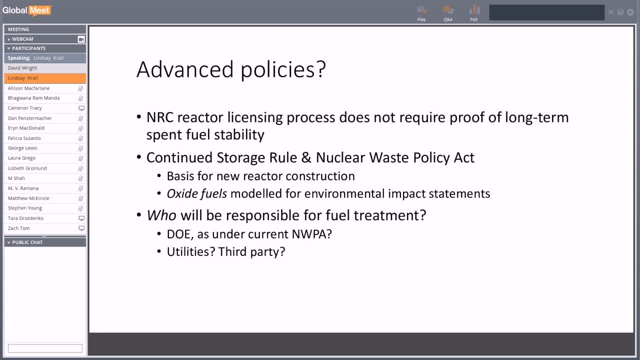 You can build nuclear reactors even though we don't have a waste disposal program. However, for the environmental impact statements that support the proposition that the fuel can be stored safely on the surface and in a geologic repository considered oxide fuels. These were modeled in the simulations of fuels. 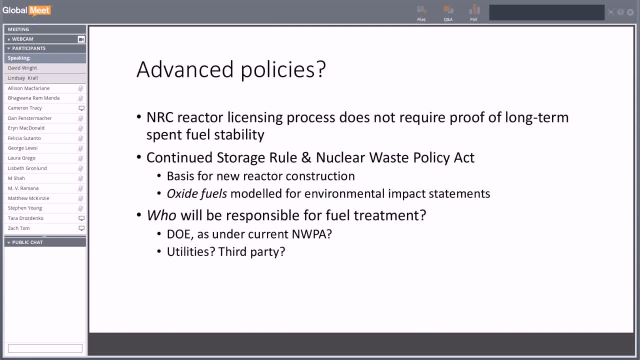 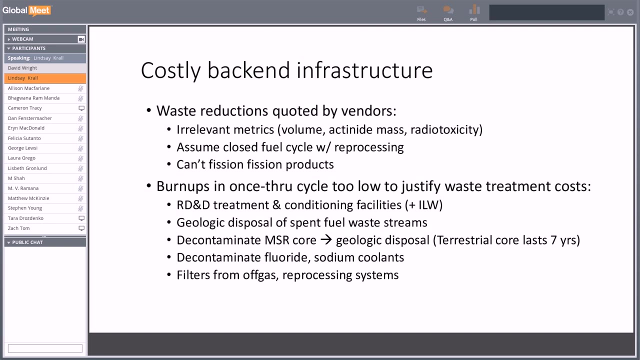 They're very high at the level of the prevention of higher-level emission. Anymore questions? I'm trying to read my response. I don't think I have anything else for you. I had another question. The waste reduction that the vendors are quoting use irrelevant metrics. 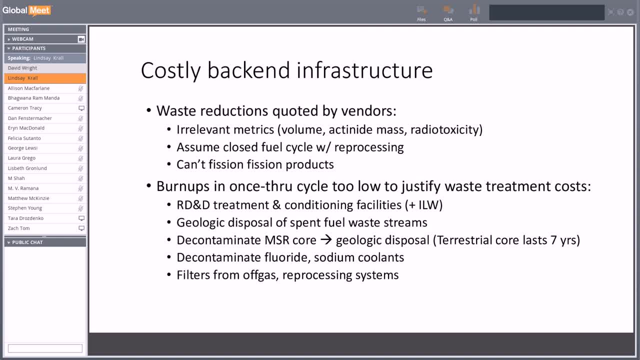 They're formulated around volume, actinide mass and long-term radio toxicity, whereas in the geologic repository back-end aspects we're more interested in the mobility of radionuclides in the environment, the heat output as provided by the fission products. You also need to process. say, even if you're left with a mass of fission products, those are still going to be needed to be put into some sort of stable matrix, such as in France. those are vitrified, so ultimately you have a larger volume of materials. 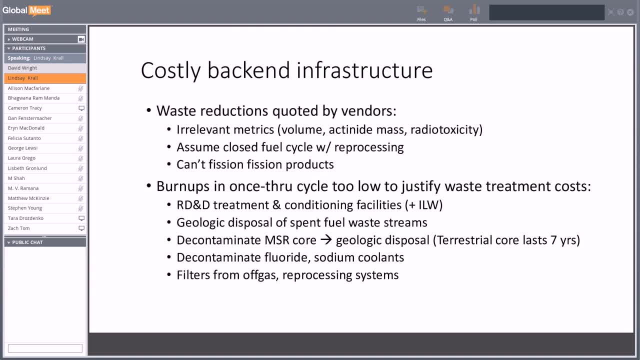 In addition, the metrics assume that closed fuel cycles with reprocessing are adopted and since you can't fission fission products, then, as has previously been determined a number of times, advanced reactors will not obviate the need for geologic repositories. 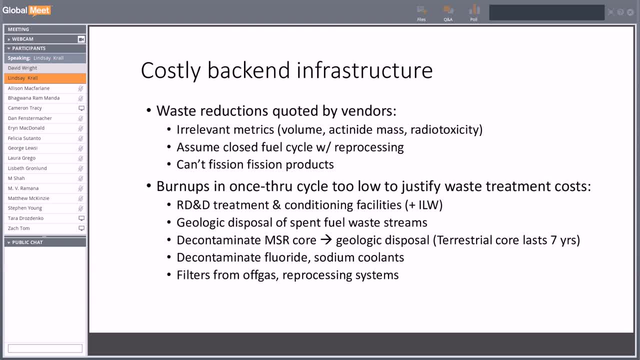 If the advanced reactors are deployed in a once-through fuel cycle, probably the burn-ups will be too low to justify the bloated waste treatment costs. There's going to be RD&D required to develop the treatment and conditioning facilities, and then these facilities are also going to generate intermediate-level waste that needs. 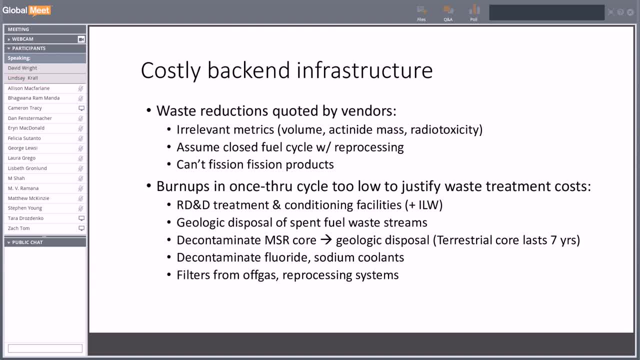 to be disposed of. In addition, the cores of the reactors need to be decontaminated. For instance, the molten-salt reactor that has all the radioactive material dissolved directly into the coolant is just going to be coated with radioactive elements. so these 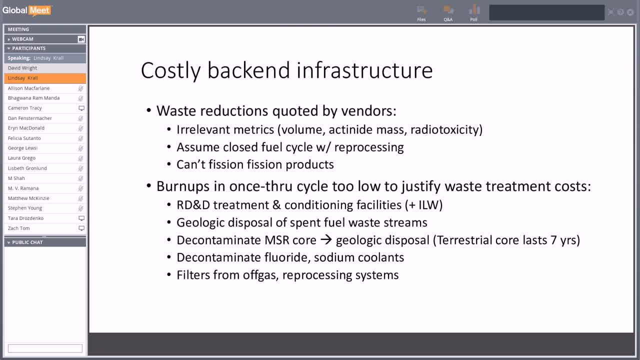 cores will need geologic disposal. Terrestrial Energy, a Canadian company, is promoting cores that only last for seven years, so it seems that there are going to be a lot of cores that need to be disposed of. It's not really clear what Terrestrial plans to do with the core after they remove it from. 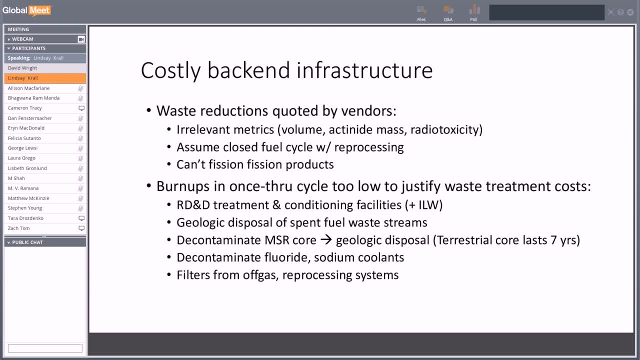 the site. But anyways, you're also going to have to be careful. You're going to have to be careful. You're going to have to be careful. You're also going to need to decontaminate the fluoride, salt and sodium coolants with. 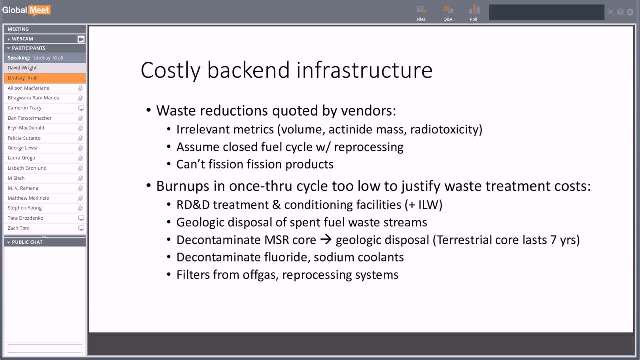 water-cooled reactors. This is pretty straightforward because you can just filter the water and remove most of the radioactivity. but fluoride and sodium are going to require much more intensive chemical processes. And then there's filters from the off-gas systems. You're going to have to be careful. 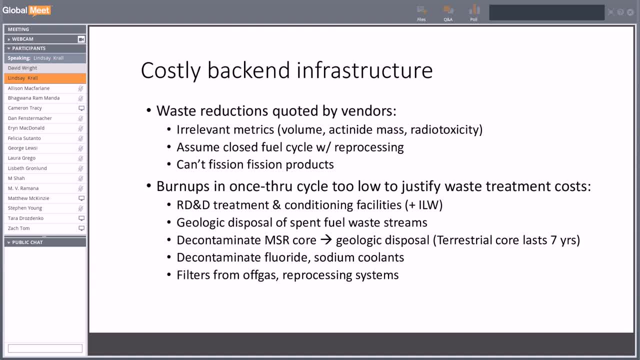 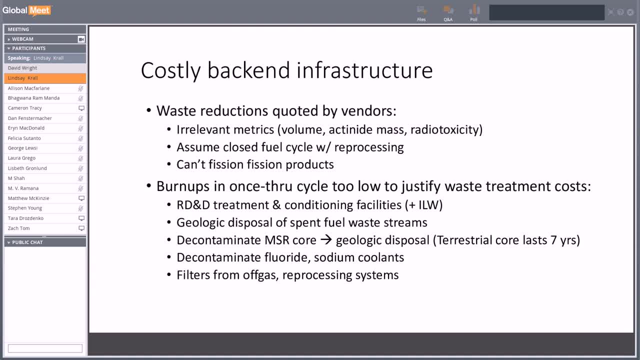 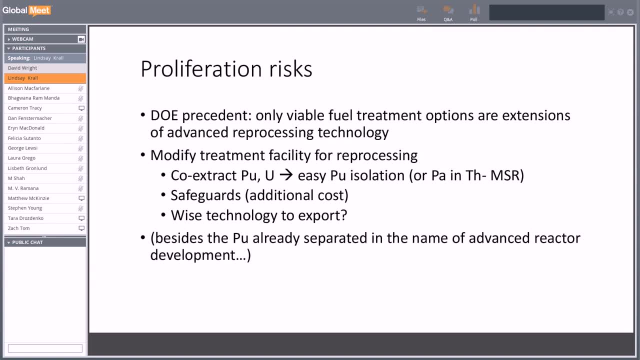 And these filters are going to be classified as high-level waste, Not to mention the proliferation risk. It's kind of concerning that the DOE set is left in the outfields. It's not just for salt, Not just in the outfields. 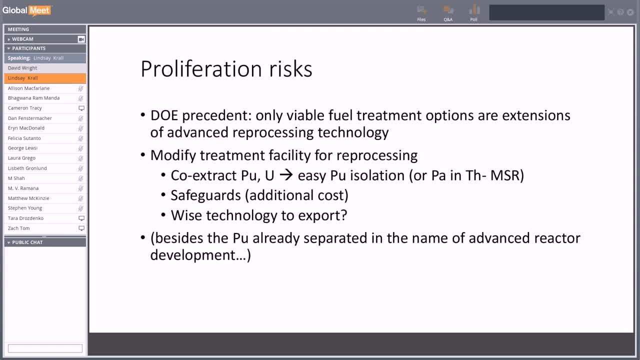 this precedent that the only viable fuel treatment options are extensions of advanced reprocessing technologies. They've already proven that it's pretty easy to modify these treatment facilities to reprocess the waste or extract fissile material. So you can- either you can- co-extract plutonium with uranium as opposed to in a once-through-fuel cycle. 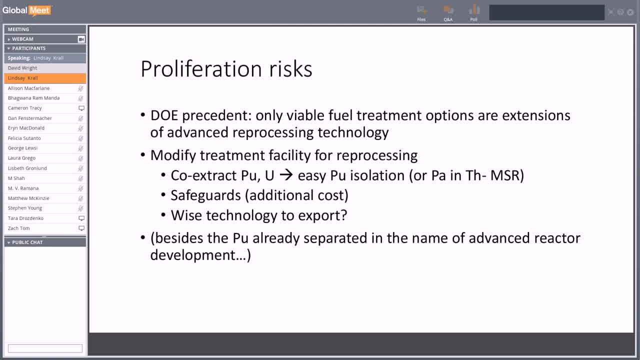 say, GE would suggest that the plutonium remains with the fission products in the salt bath, the pyroprocessing salt bath. But by just changing minor aspects of the chemical conditions you can co-extract plutonium with the uranium And then this would be pretty straightforward to separate from the uranium and you have 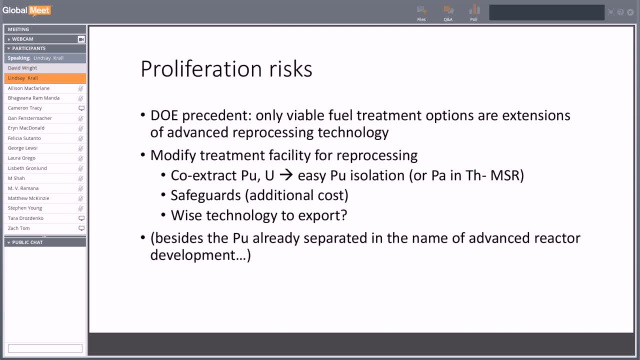 a weapons-usable material, So safeguards are going to be an additional cost, and no one's really asking whether this is a good technology to export. Well, a lot of people are asking it, just not the policymakers that are funding the reactors And all these other things that we're going to be talking about in the next few minutes. 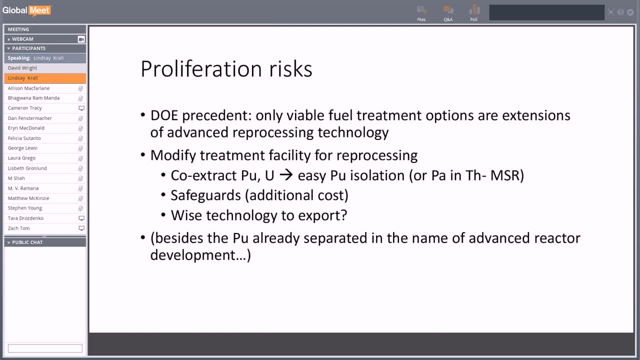 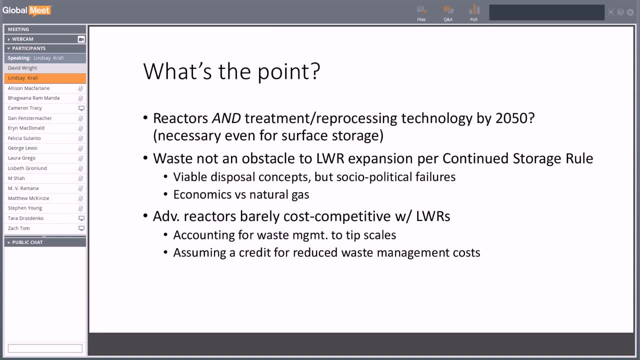 these proliferation risks are in addition to the plutonium that's already been separated in the name of advanced reactor development and needs to be dealt with. So is it really likely that these reactors and treatment slash reprocessing technologies will be available by mid-century? It's kind of an issue that the treatment and reprocessing is not only 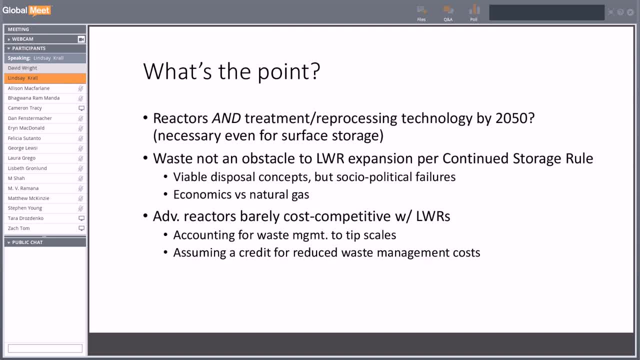 needed for the geologic disposal, But they'll be needed to just secure the waste at the surface, because all the fuels are violently or really easily dissolved by water or they can burn. So it's also worth pointing out that waste isn't an obstacle to light water reactor expansion. for the continued 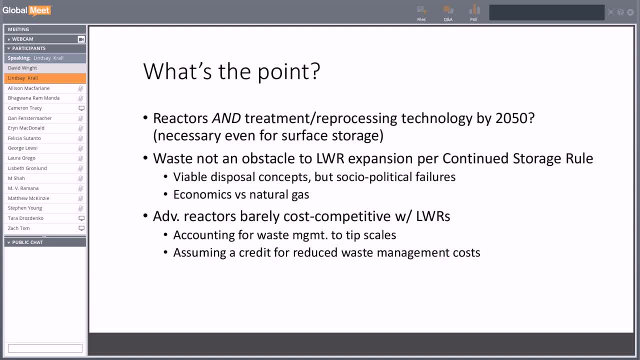 storage role And there are several viable repository concepts. but there have been social political failures that some countries have not surmounted. Also, the economics of nuclear is challenged by natural gas, And advanced reactors at current estimates are barely cost competitive with light water reactors. 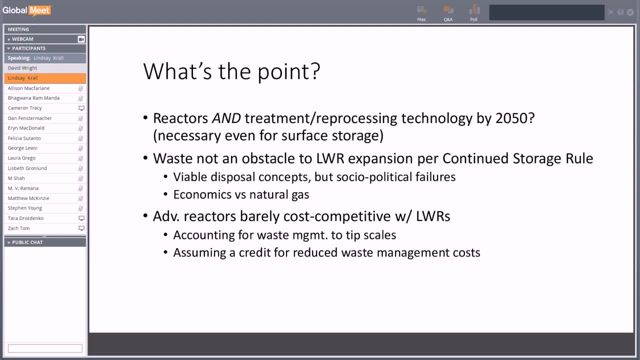 But if the waste management costs were to be considered then they would very unlikely be competitive. A lot of the vendors are actually assuming that they'll get a credit for reducing waste management costs. That is, they expect the DOE to pay them to collect the spent commercial reactor fuel. 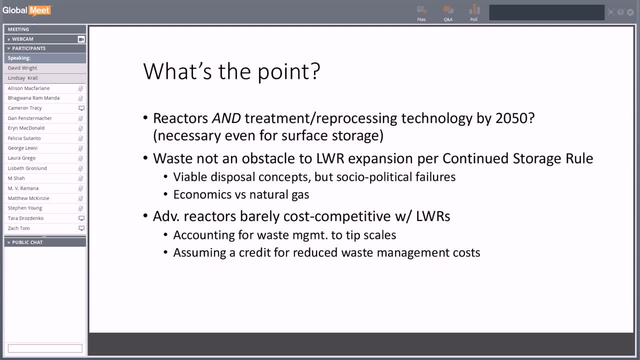 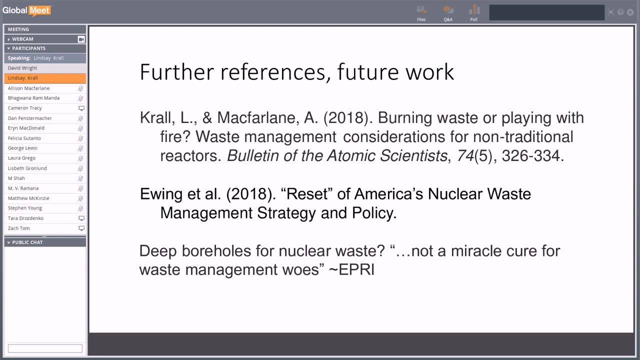 that is currently available. Prior to that, they would have to pay the company for the entire cost of the gas. So that's something that's a positive. Okay, So references for further reading. This presentation was made from an article that was published in the autumn. 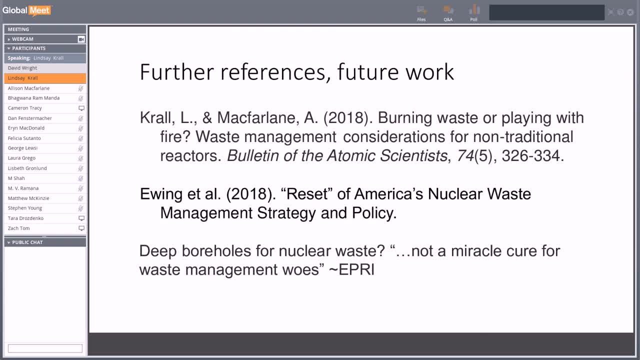 And also there's a new report out on the research. This is a new report. It's written by Dr James Herring, who is a professor at the University of Northern Michigan. One of the other papers I want to share with you is the one that was published in the autumn. 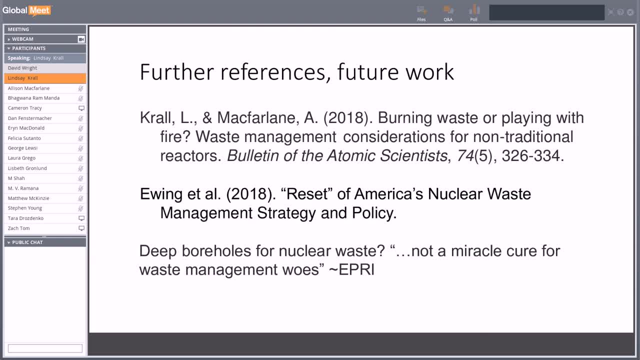 This was published by Dr James Herring reset of America's nuclear waste management strategy, and this has a lot of good pointers for how a geologic repository program might be restructured so that it can be more successful, and I'm also looking into deep boreholes for 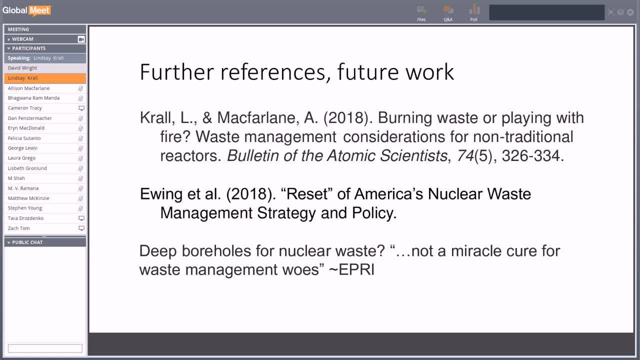 nuclear waste. the vendors that have acknowledged that they'll produce high level waste suggest that they can easily deposit the high level waste on a deep borehole. but to state it simply, this is not a miracle, miracle cure for waste management woes, and that was said by the Electric Power Research Institute. 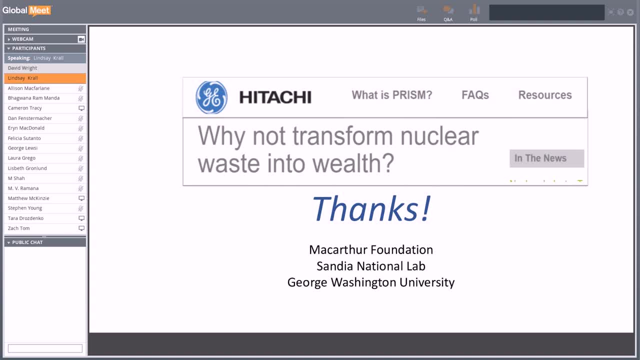 okay, so you tell me why not transform nuclear waste into nuclear waste and how can we do that? well, and many thanks to my funders and George Washington University, and I also benefited from discussions with the researchers at Sandia National Lab, and I'd be happy to take any questions. 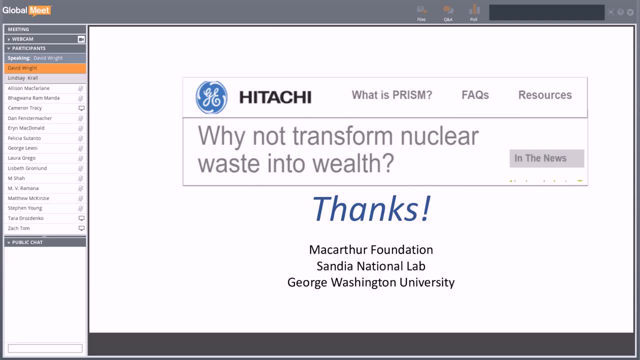 okay, thank you. we've got about 10 minutes and I noticed that Ramana has a question. we'll get to him in a minute. if if others have questions, let me know. I wanted to start out with something that, given the problems that you've talked about here with the with waste, with non-proliferation concerns- 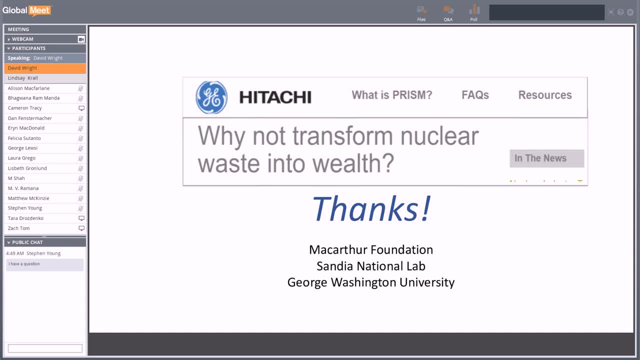 things like that. it's a little surprising that that these just that there's so much enthusiasm about these systems, and I'm wondering if that's partly because they're still early enough in research and development that people are simply arguing that those problems will be solved eventually. 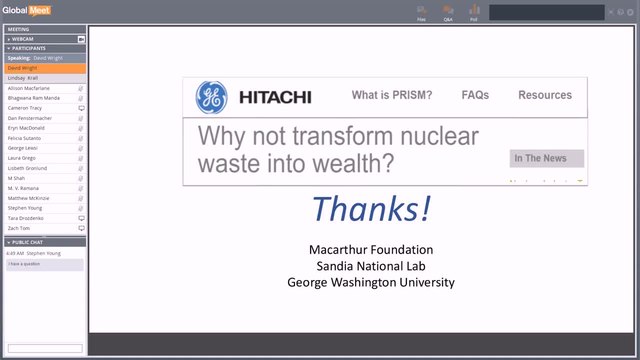 and that the benefits will outweigh the those problems. or I mean, what's the dynamic, that sort of pushing these ahead? I think there's a great fear that the nuclear enterprise is going to collapse due to the major economic issues that it's facing. so, you know, Westinghouse has declared bankruptcy and so a lot of. 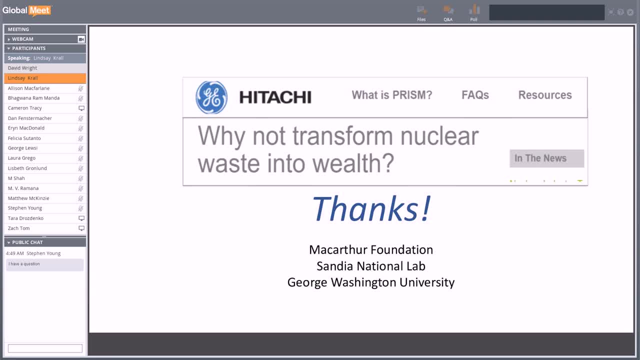 this is, like you know, saying all light water reactors are unsafe, they have all these issues and so these advanced reactors are better than light water reactors in all these respects and like, if you look at design basis failures for light water reactors, then sure, maybe there are some benefits to advanced. 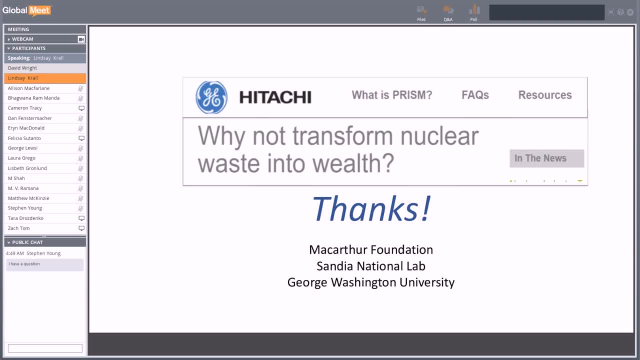 reactors, but there are a lot, of, lot of, you know- aspects that just aren't considered in their- like you know- engineering for their safety. And then, from the policy side, I think there's a lot of motivation to be like competitive with, say, China and Russia and sort of put an advanced reactor to market. 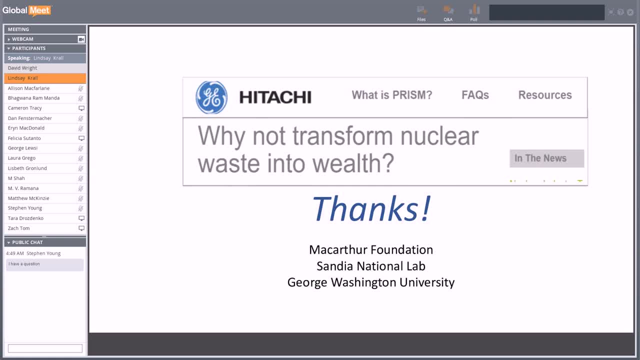 before you know the other countries. So there's a competition aspect And there's a hope that, like developing countries, will adopt nuclear, because advanced reactors are saying that they're plug and play, So you can just build a reactor and then it operates itself. 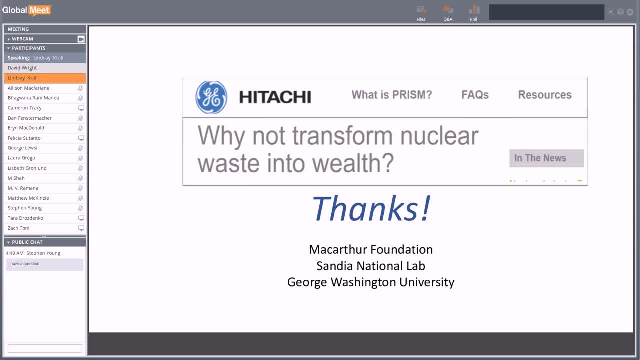 So, yeah, it's a pretty, it's not about climate, Climate change. I guess you could say: Okay, Let's see, Ramana, I've just unmuted you. Do you want to ask your question? Sure, Hi, Lindsay. 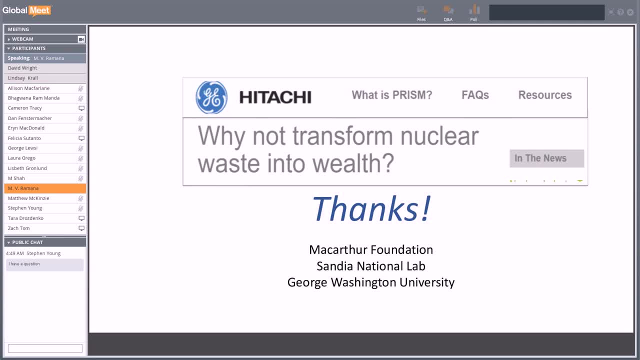 Hi Ramana. So as much of what you've said is based on US regulations for dealing with waste And I was curious how other countries might deal with these new waste forms and if their regulations are Easier to deal with or more difficult. I know that you know, you have a lot of experience. 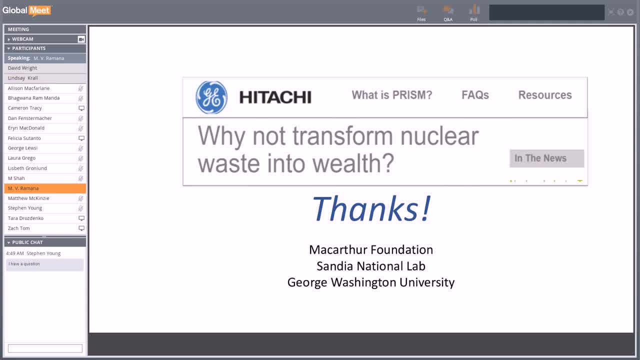 with Sweden. So any thoughts on that? Well, in Sweden, let's say, there's more accountability for the implementer of the waste management program. So let's say Vattenfall, the Swedish utility. they are the implementer for the waste. 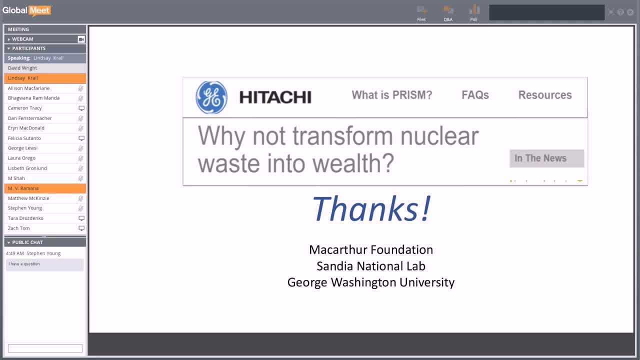 repository, rather than say the government Right, As in the US. So when you have the utility needing to think about how to deal with the waste from advanced reactors, then I think if they're going to be held accountable for the waste, then they're. 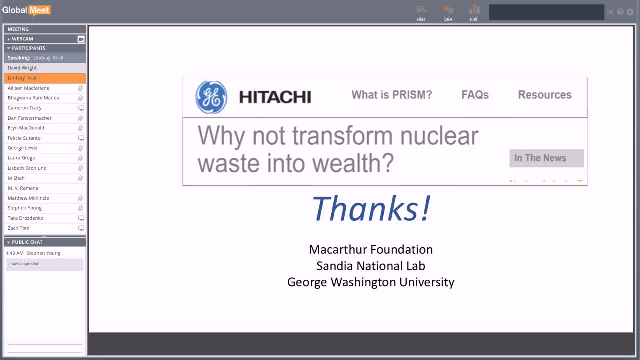 going to be more realistic about what is going to be required to dispose of it And they're going to, you know, like in Canada as well. this is the case, And the Nuclear Waste Management Organization does that Right- reviews advanced reactors every year and they compare it to what's required for. 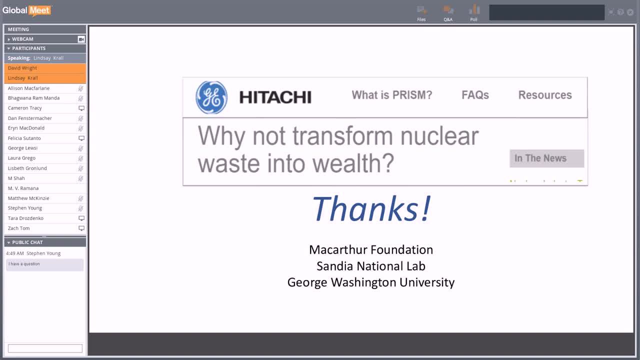 repositories for oxide fuels and it's not clear that they'll be willing to build an advanced reactor. and in addition, like the other countries that are developing the sodium fast reactors, they're using mixed oxide fuels as opposed to the metallic fuels, so probably mixed oxide fuels will be easier to dispose of in that they are not flammable, although there are. 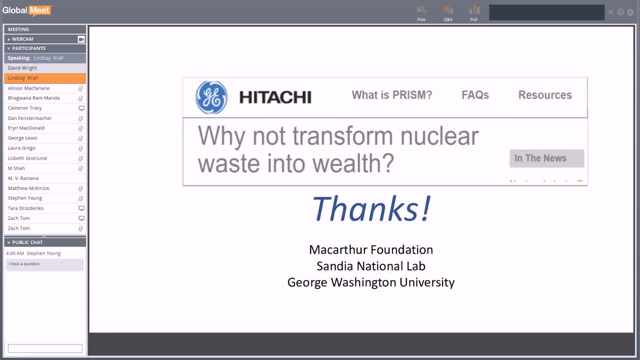 some potential. you know, mixed oxide fuels are not necessarily preferable to pure uranium oxide fuels. so yeah, internationally, i think. yeah, my question was also in the in the safety realm, when it comes to licensing reactors, there's an argument that many of these advanced reactor vendors offer, which is to say the nrc is exclusively strict. they have this very they're. 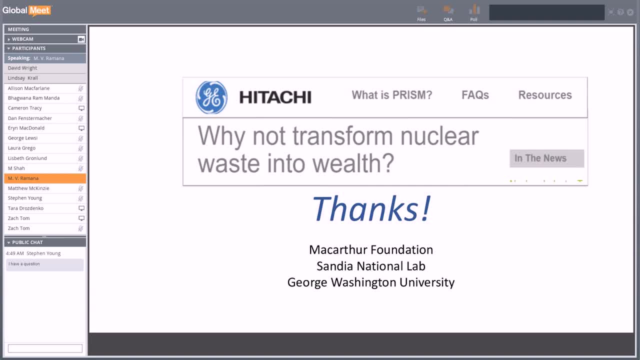 only geared towards light water reactor licensing and so on, and therefore we know we need a more flexible regulation regime. i'm wondering whether there's a similar kind of comment made about the waste regulations for the, whether the regulation scheme in the us is quite strict um. 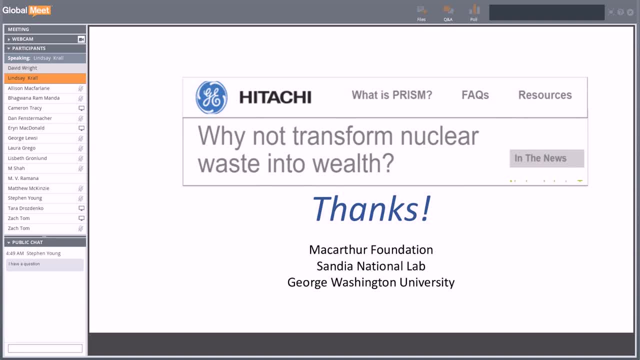 uh, i do not think the waste regulation um in the us is more strict than elsewhere. okay, okay, yeah, we can. we can call for a plan, okay, um, stephen young, you had a question, stephen. uh, thanks, lindsay. um, so let's pretend that you work for the congress and you are the key. 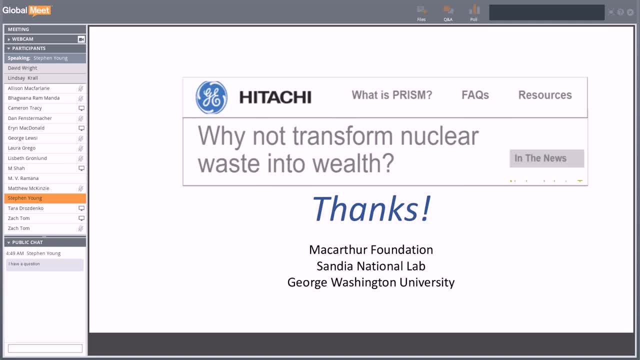 appropriations staffer who gets to decide how the doe spends, say, a billion dollars on nuclear power and you can spend it on any piece of nuclear power equation, on safety, on disposal, on advanced reactors. how would you spend a billion dollars on nuclear power if you were a doe? you can fund other companies. you can fund private business. you can do whatever you want. 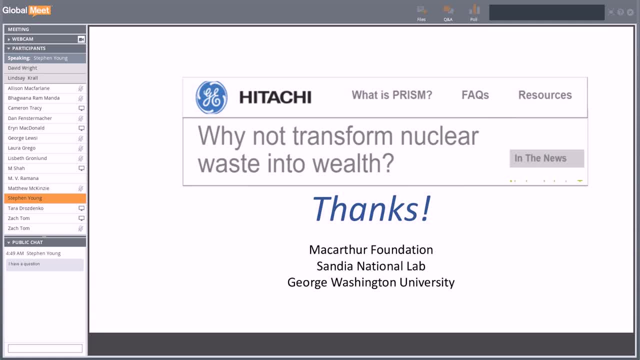 with that money? what would you do with a billion dollars for nuclear power research? um, i mean, i would. i would look into the geologic disposal. i guess. try to fight um more. you know appropriate repositories and um, but at the same time the doe doesn't really have. 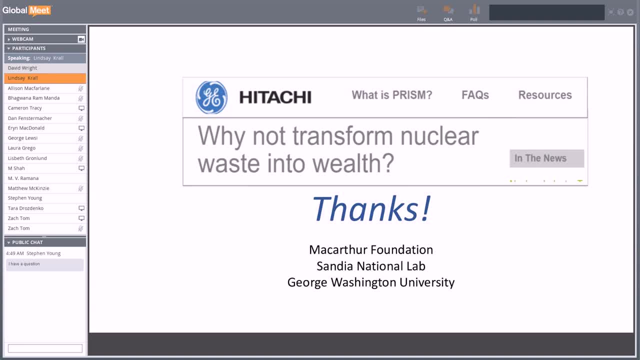 that choice. so i would encourage congress to, you know, look more closely at the nuclear waste policy act and see if we can re, um, reset our program so that it can be more um successful. you know, looking at the successes that have been experienced in other countries, um. but i mean, yeah, there was unlimited money to spend on energy research. i think an easy way to. 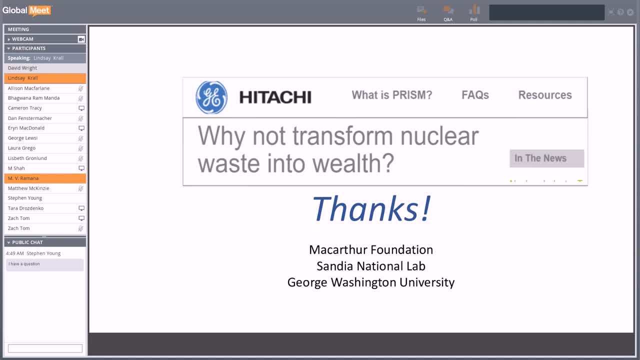 get. that would be from the defense, um, defense spending. that's where most of the research money goes, so not really into energy. so, um, steven, i assume this is not a a purely rhetorical question, that that there are people and the appropriations are going to be looking at this. yeah, and and the 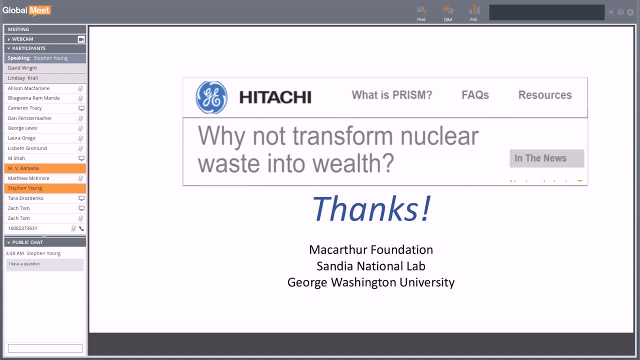 questions are: how much should we be spending on advanced reaction research versus safety, versus um disposal, r d funding and the other questions that are: more that? would you get more value for your spending? okay? um, well, i think that light water reactors are um sufficient and, yeah, you can. 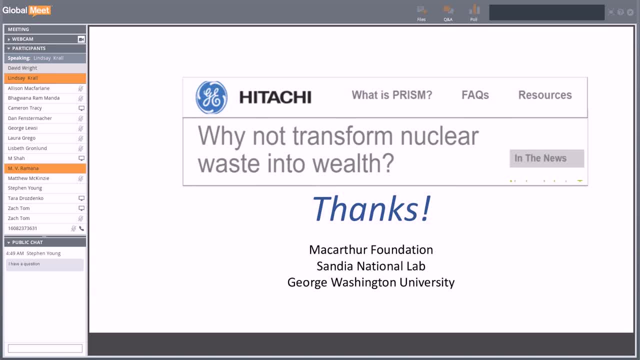 study ways, there's still a lot of progress that can be made- and that you know those technologies pertaining to fuels that are more? um tolerant of accidents and you know lower dissolving than uranium dioxide fuels, um. so i think, if you like a lot of the advanced reactor motivation is to make. 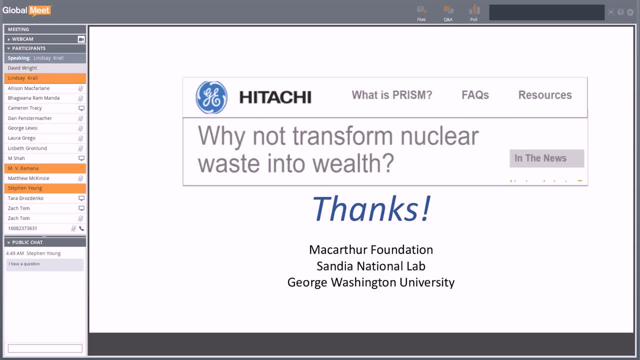 questions about that um, and i think that it would be useful to do that um, but also having um these uh questions and the substitutions. i don't have a link to that in the chat box, um, but i think you know it's a good thought to do that, but i think to do it, uh, looking at. 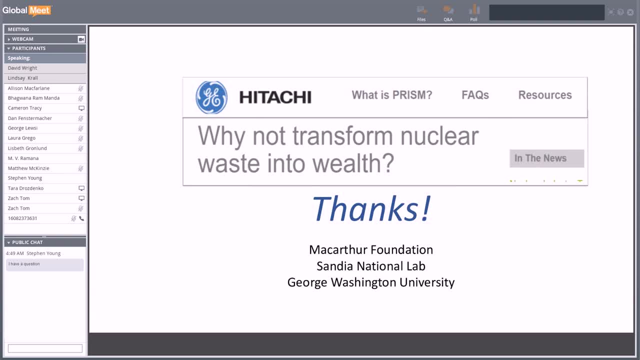 the results of the research. i think the most important thing is to be able to do that, and i think that's a good point. um, You had mentioned that Yucca has an oxidizing chemistry in the ground, which surprised me given some of the things you had said. 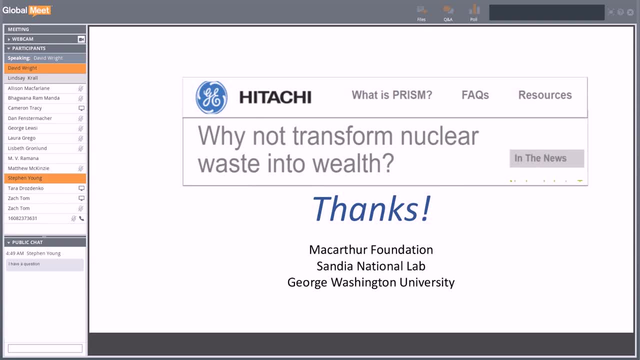 Can you say something about how that was chosen, how that decision was made? It doesn't sound like the environment you would like to have for a repository. Well, the decision was made by Congress, you know, and not the technical experts. So I mean, this was in the 1980s. 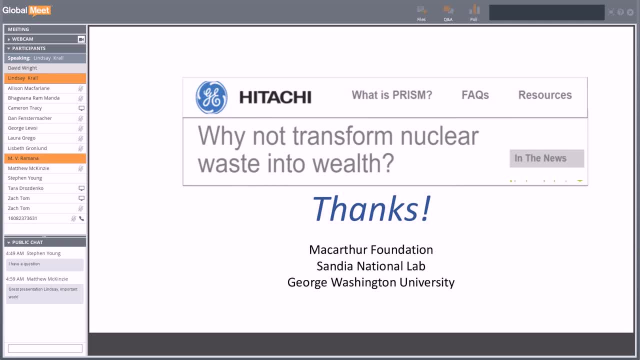 It was before a lot of the research on nuclear waste disposal was conducted. Like the natural analogs, a lot of that work was done in the 1990s, So maybe in the 1980s it wasn't, you know- appreciated how much an appropriate 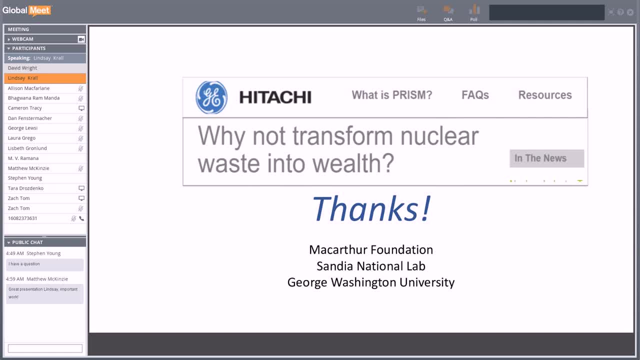 geologic environment can help you. Okay, and this was also before, like the more successful concepts were introduced. So there were all sorts of different ideas being thrown around and the US sort of went full force at one idea without really you know: diversifying a research program. 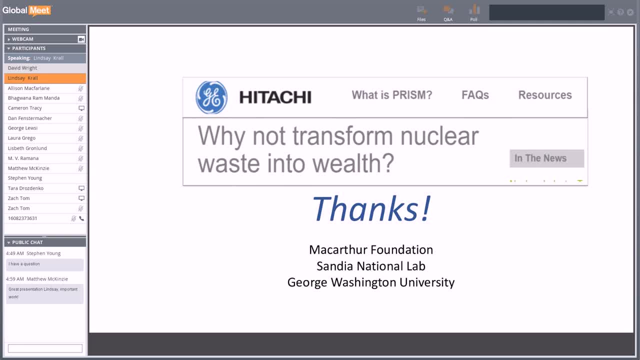 And you know it was politically motivated And Nevada had it was pretty weak politically. So it sounds like part of what you're saying is that the understanding of the science has moved on since that decision was made. But given the oxidizing environment, do you is that a particularly bad issue that people now have to reconsider? 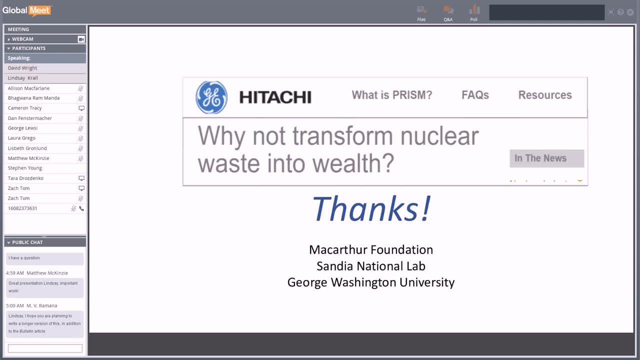 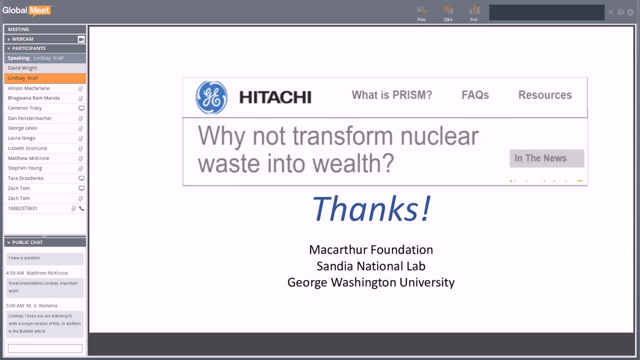 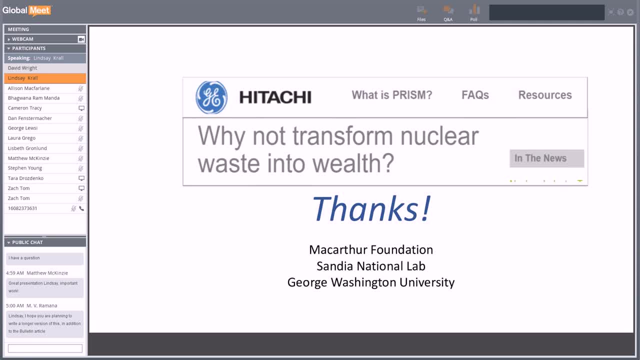 over the long term. You know you can't really refer to natural analogs and you know, at first it was thought that yucca mounted mountain had really really slow groundwater flow rate, but as the project progressed they realized they were faster than expected. so that made the oxidizing, the corrosion. 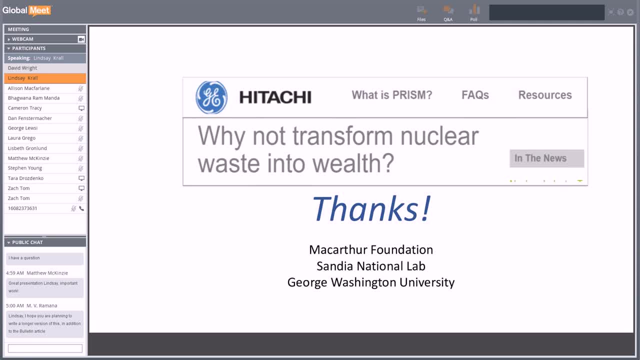 occur faster from the faster water flow rate. We ended up just with a really really engineered repository design. They had to introduce a titanium drip shield just so the dose regulations could be met, and the drip shield is absurdly expensive. It's kind of a joke in the international community how expensive it is. 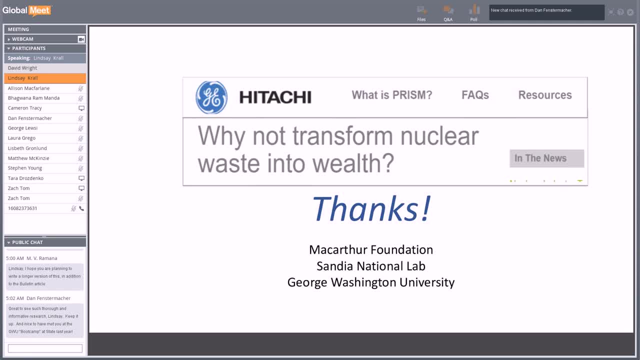 Say you have an oxidizing environment. if you want to prove long-term safety, then you're just going to have to spend a lot more money if you're not getting passive benefits, Okay, well, thank you very much. Ramana is encouraging you to write an even longer article than the Bolton article and 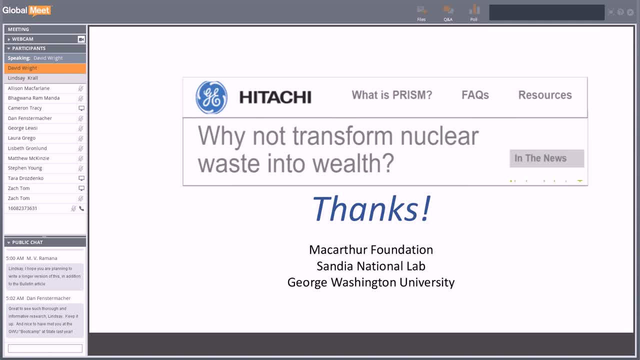 I think that getting this discussion going is obviously important, so thanks again, and we will post a recording of this for people that weren't able to make the talk today. Okay, Thanks for organizing this, David, and thanks everyone for tuning in. 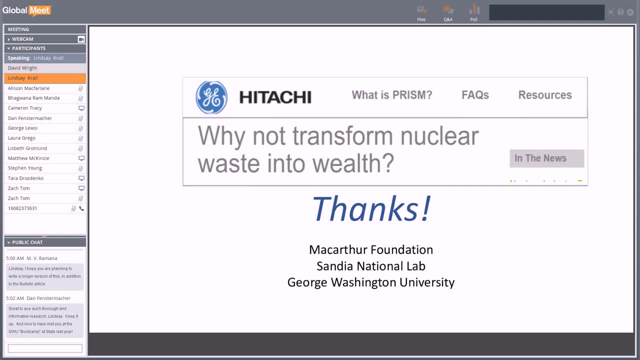 Okay, Goodbye, Bye now. 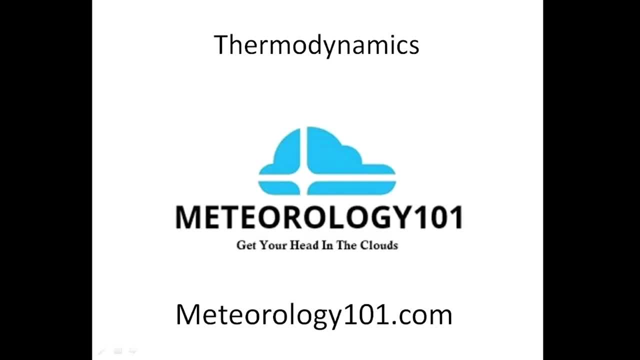 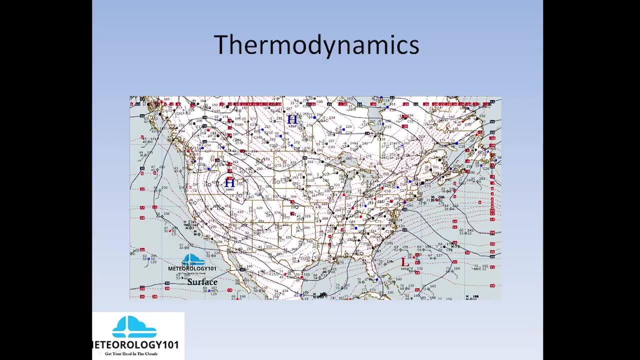 Alright, welcome back to Meteorology 101.. In this video we're going to cover thermodynamics. Visit my website, meteorology101.com. A lot of info over there And please comment on these videos if you have any questions. So let's get started. Thermodynamics- pretty much what we get out of a sounding is- and weather observations- We covered weather observations in the last video. And all that's put into a computer program and we get the big picture of what's happening with weather systems. 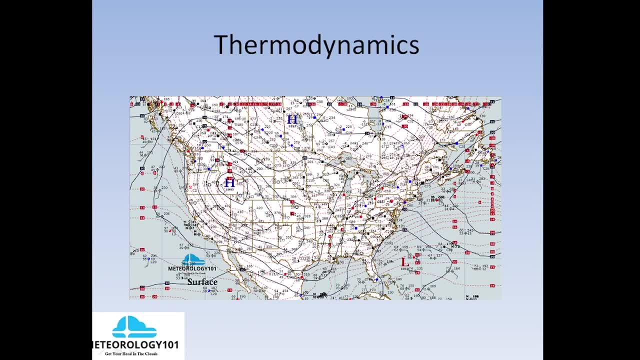 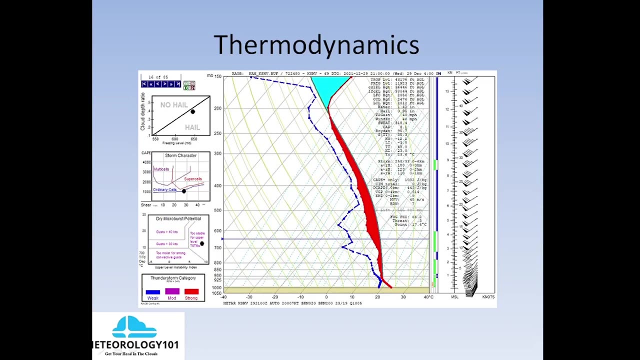 So with thermodynamics, we use those tools, such as a sounding, to get the upper layer charts. We may jump into them if we have time, but we're going to try to stick to the course. So soundings, The thermodynamic tools that help weather forecasters, answer the questions of what's going on in the local atmosphere. 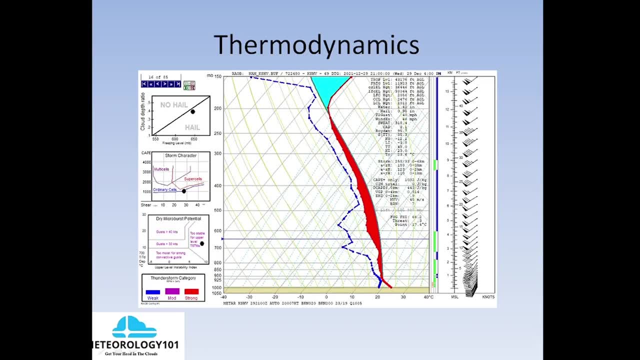 When they let a weather balloon loose, the radio sound goes up, sends back data mandatory levels and then it has the option to send back essential data at any level in between. So The mandatory levels are 1,000 millibars, 925 millibars, 850, 700, 500, 400,, 300,, 250, and 200 millibar levels.